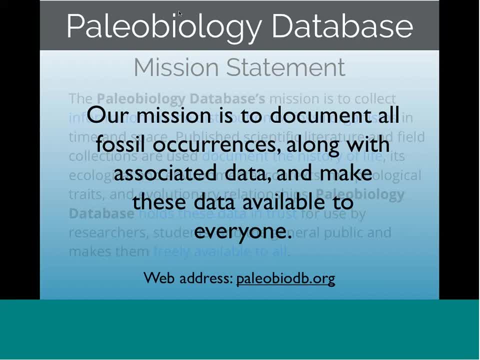 So you can see here on my first slide the real mission statement is kind of grayed out in the back. It's kind of long, but really our mission is to document all fossil sciences on the planet, along with other associated data, and to make these data available to everyone. 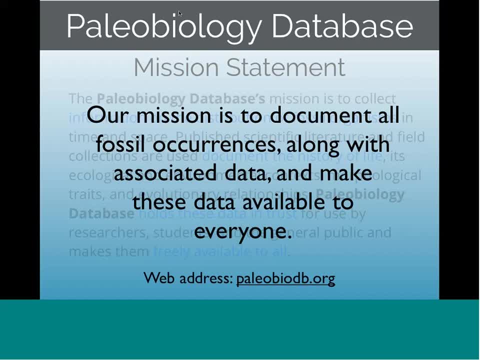 And so we've been striving in recent months and years to really hit that last one, make those data as publicly accessible as we can, and I'll show you some new ways we've been doing it. If you've never been, the website is down here at the bottom. 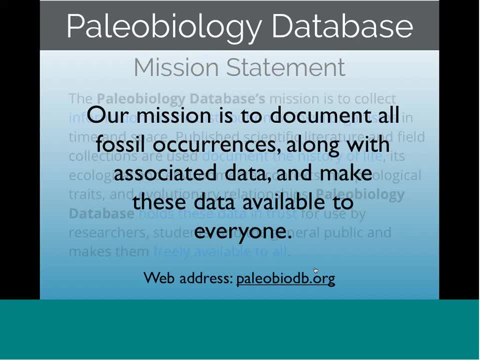 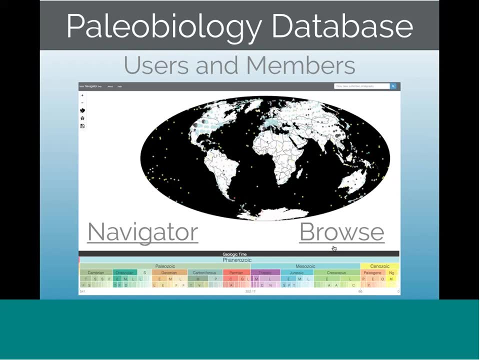 And I'm going to be bouncing back and forth between this presentation and the website, so it may be easier just to watch and then go check it out yourself later. but that all means if you have questions, type them in the chat and we'll answer them when I'm done. 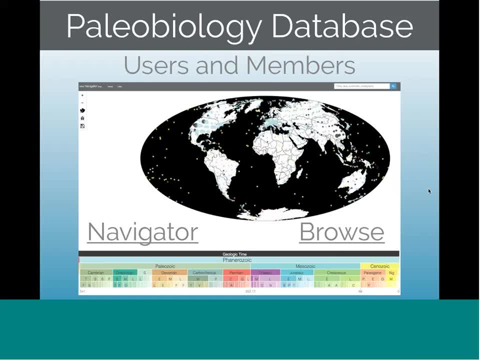 So one thing I want to stress is that there are basically two kinds of people who use the database. One are just users. Since we make all this data available via the web, you don't have to be logged in or signed up or be a member of the database to utilize it. 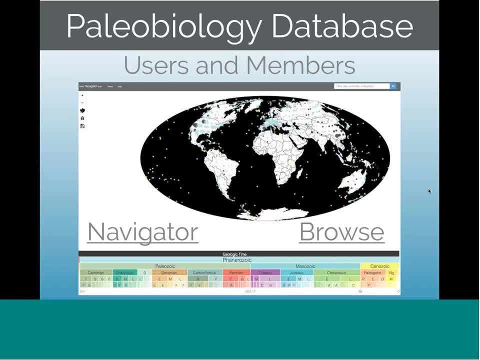 Okay, So virtually all the data that's entered is as available to people logged in as not logged in, And I will show you the difference between the two. So we recently launched a new tool called Navigator, which is a data visualization and accessing tool. 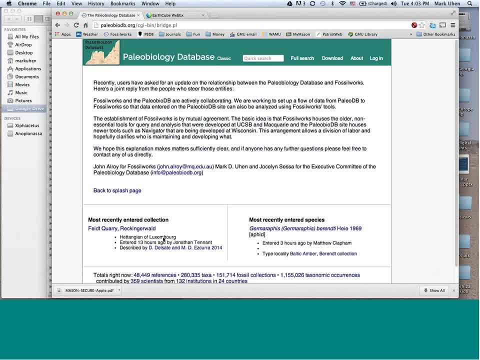 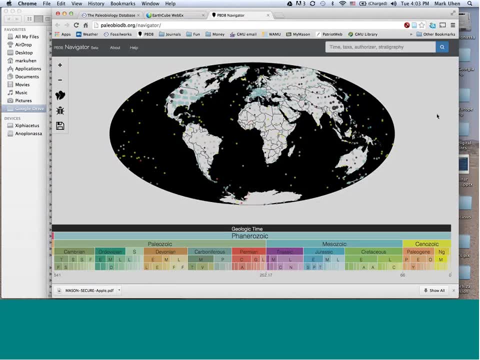 So we'll go check it out right now. So here it is. It takes a little minute to line up. I'm going to get rid of this stuff and go straight to it. So it shows you the world and you can – it visualizes all the data in the database at 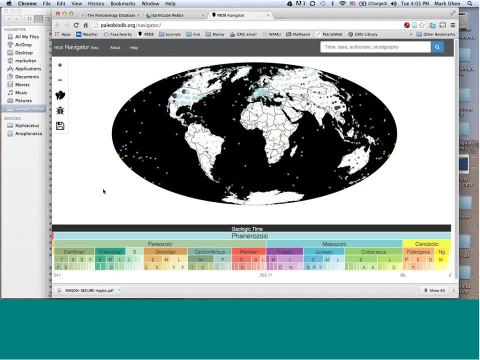 first, and all those dots represent different clusters of collections. so bigger dots mean more collections, smaller dots mean fewer collections, And you can use the map, these tools and this time scale to zoom in on exactly what you want. So, for instance, if you wanted to look at fossils destined in Jurassic, if you click. 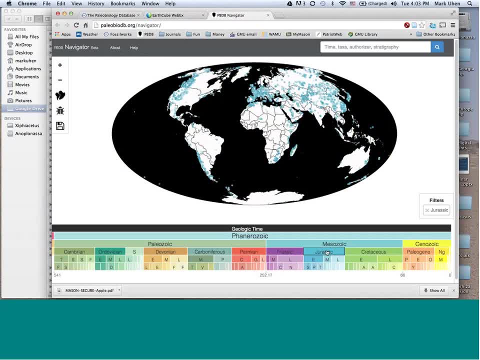 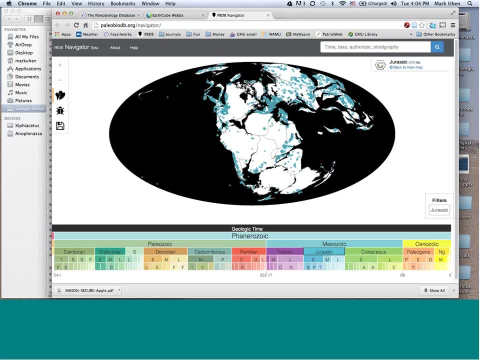 on Jurassic note, all the dots change to this pretty blue and even shades of blue- early, middle and late Jurassic. And if you want to see them in the Jurassic, you can click here and reconstruct it to the Jurassic. That's all Jurassic fossils. 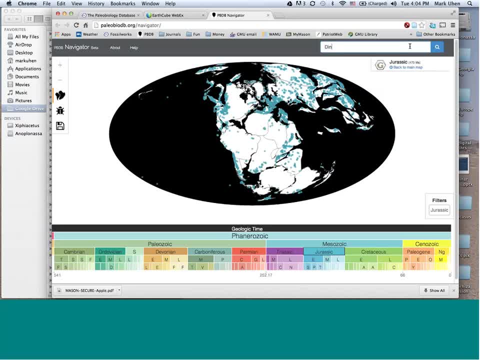 If you want to see a certain taxon like Dinosauria, you can do that, Select it and boom. now you have all Jurassic Dinosauria reconstructed in the Jurassic, And the thing to note about this is these maps are being drawn dynamically. 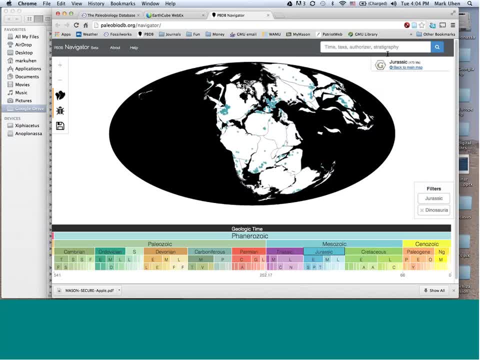 The paleo plate positions are drawn from G-Plates, a different web service tool, and the data are being drawn from the PaleoPlate And you can even click on them. see a little bit down here in the corner. oops, can't do. 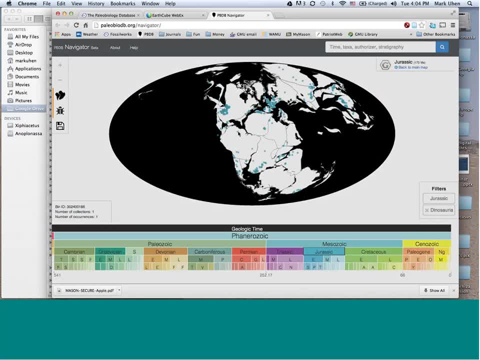 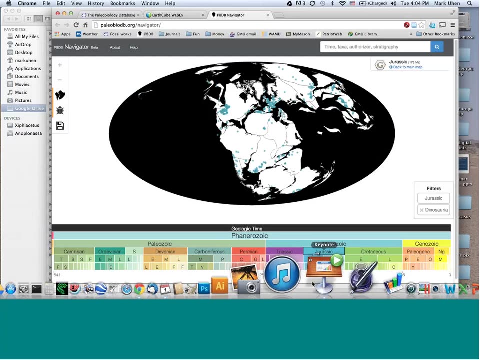 that about it and you can click and get a little bit more information, And if you wanted to, you could in the end hit this little disk icon and download the data that's shown on this map. So that's one way you can interact with the database without ever being logged in at all. 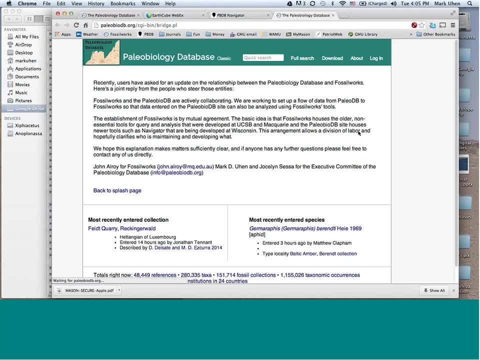 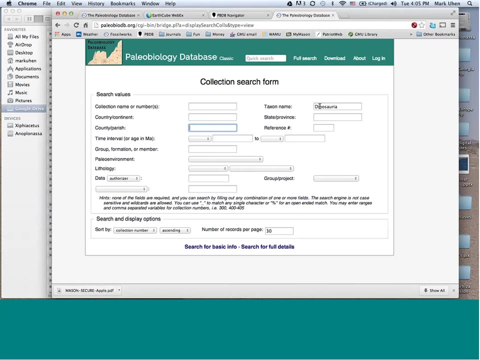 You can also simply just browse the data. So if you get to this screen- This is a not logged in text interface- You can go here and see exactly the same data. So here it says: Fossil Collection Records. I can say: give me Dinosauria from the Jurassic. 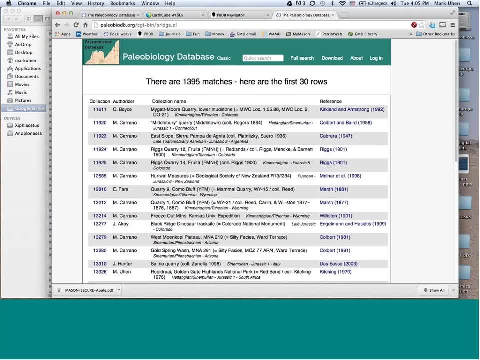 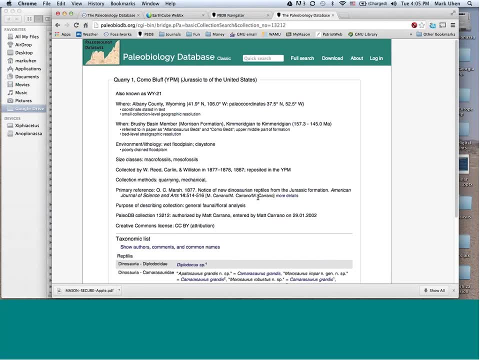 And here it comes as text, And it just comes as a list and you can drill down and see more about each of these different collections, with lots more data than you can see in the visualization. But again, this is all available via Dinosauria. 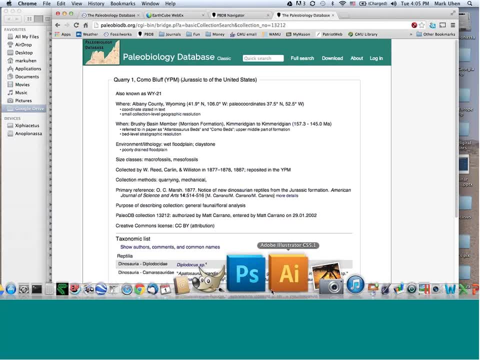 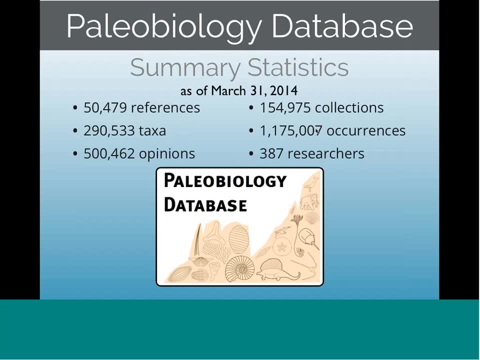 It's not available via download. without ever logging in. Let me go back to my presentation. Here's just some summary statistics about what's in the database: Lots of references, lots of collections, over a million occurrences, And you can see there that over 387 people have accounts that have entered data into. 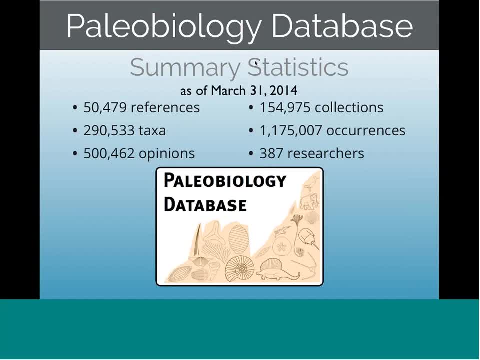 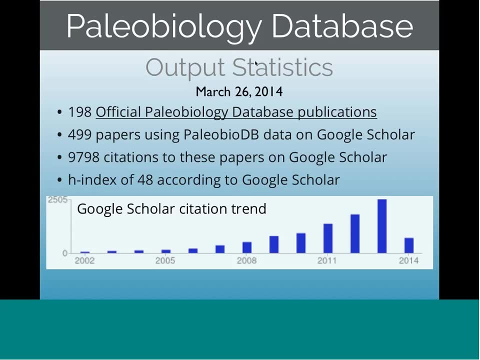 the database And these numbers change daily. So this is the numbers as of yesterday. This is probably more interesting statistics. This is output from the database, So as people publish papers, they can log them as official publications if they so desire, And we have almost 200 of those now. 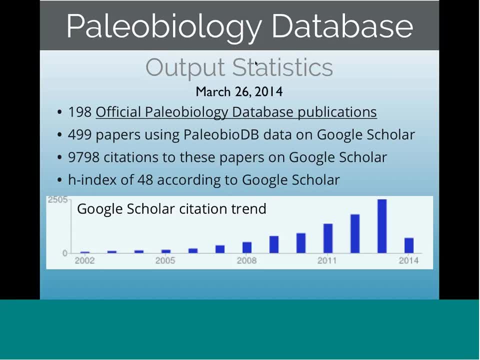 We also have had Google Scholar- look out there what papers are using the database And we have just shy of 500, probably over that, since this was a few days ago- And almost 10,000 citations to those 500 papers And the database. I'm putting that in air quotes. the database has an ACE index of about 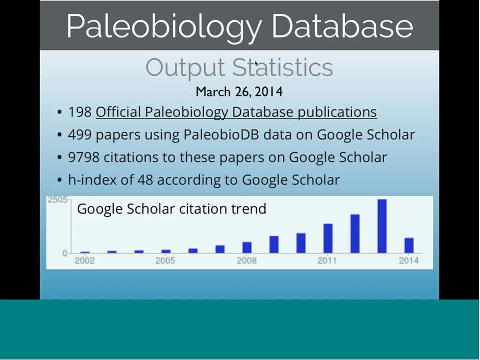 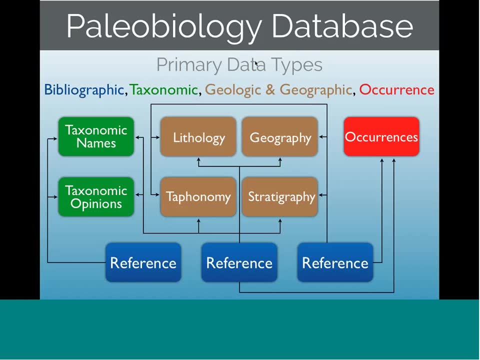 48.. And you can see, on the bottom are citations, And here there's the one that showed up in the database. The data that I just showed you was also on the list and the data that I just showed you is in the database. 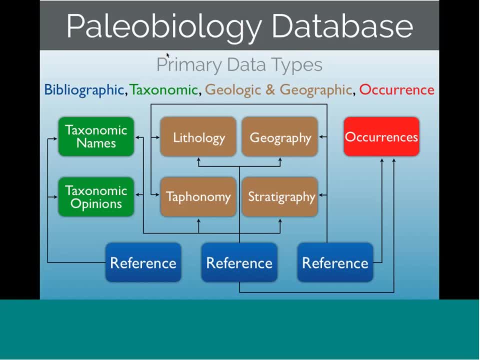 And the value of the data that's being published is the value of the reference that you're collecting and it's going to be in the database. So if you're going to look at your favorites here, you can see these three public references. 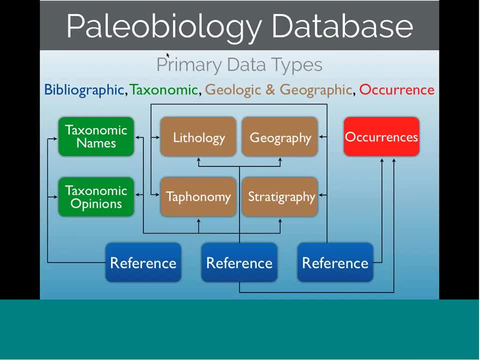 Use this before you publish as well. but in the end we need a source for the data, And that's what the blue references represent, and we have taxonomic data of two sorts, which I'll show you: names and opinions, and then a whole bunch of 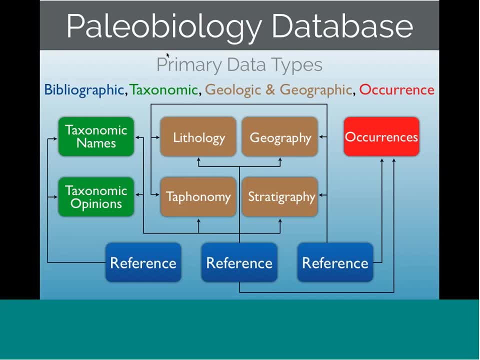 Geologic and Geographic information about mythology, geography, typonomy and satisficy, and then, in red, the occurrences themselves, And they're all. all those data types are related back to the references and there's lots of interrelationships Among the data that you see here, which I'll show you in just a moment. 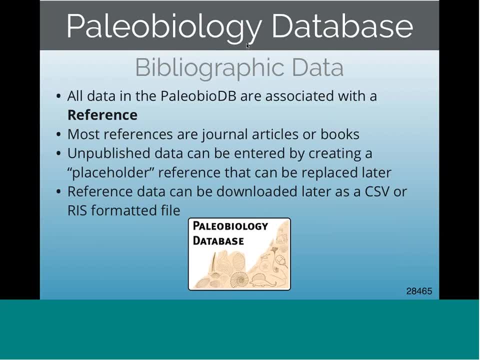 So again, primarily It's all based on Geographic data, or, sorry, bibliographic data, and mostly published works, journal articles and books. again, you can put in a placeholder for unpublished data and You can actually download all this as a CSV file or CSV file. so I'll show you how this works. 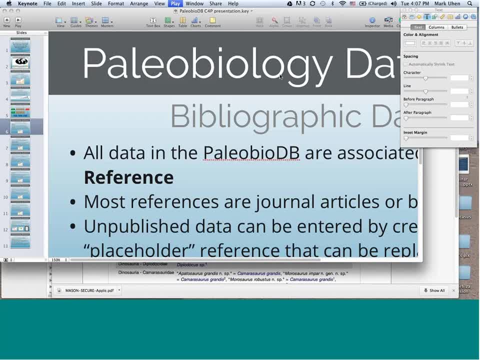 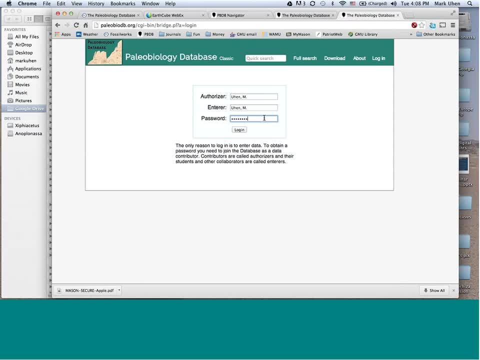 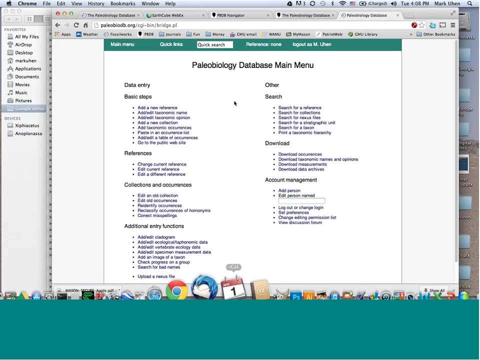 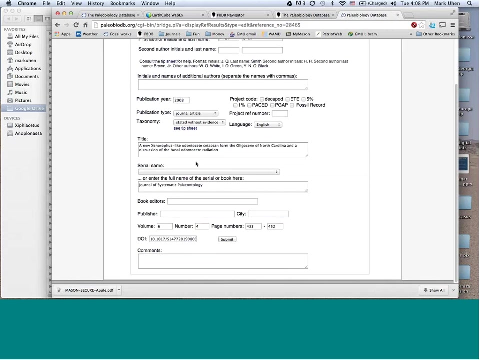 To do so I'm going to have to log in. I Think I'll get my password right and I forgot the number. So here's what a reference looks like- Basic information here- and what kind of reference when he wrote it: title and The DOI. so we're looking to upgrade this. 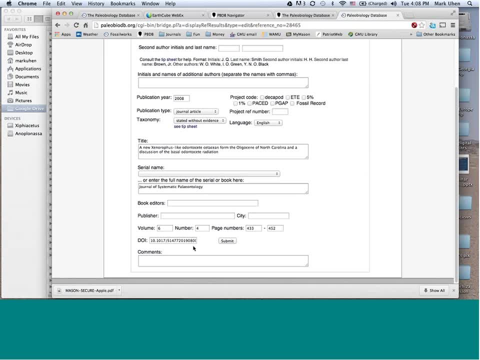 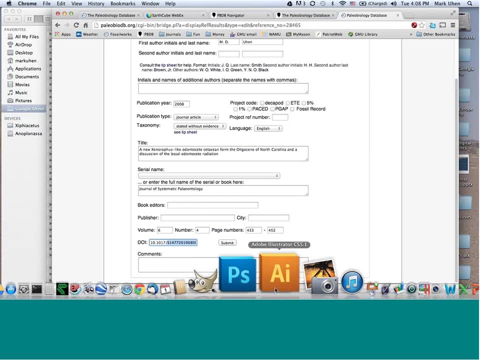 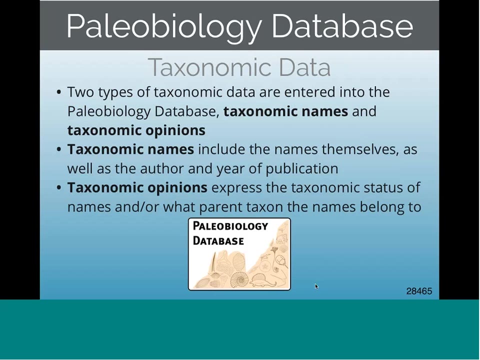 Input form in a bit and you able to just type in the DOI and have our database got the Indexes out there in the world and bringing that information for you to help save the precious. We're fun to do is streamline the user experience so we minimize the amount of 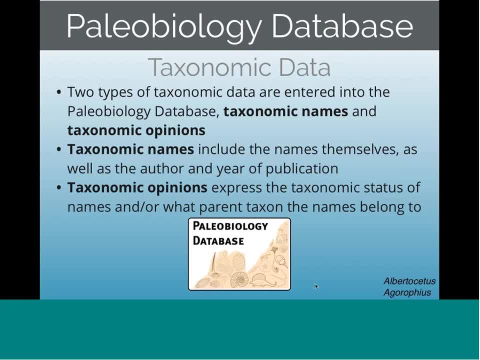 Time it takes the input data, which is will, it can be quite time-consuming. taxonomic data is much more interesting. we have two kinds of data: one on the names themselves and who names them, and then opinions about what people have said about those names. so let's take a. 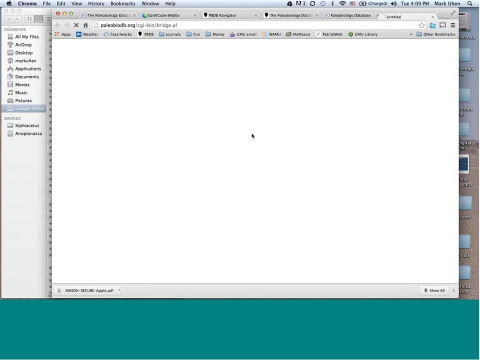 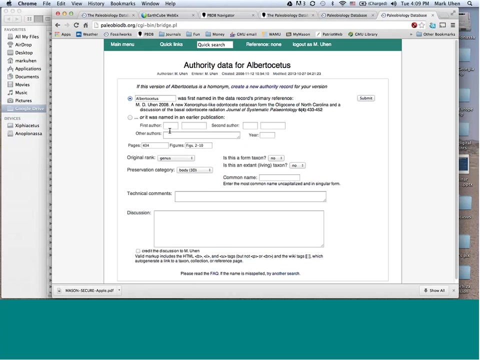 look at these two names for no particular reason other than that I'm familiar with them. so here's a name so we track who said it- this happens to be me- and- and the bibliographic information so you could go back and find the paper and find out exactly. 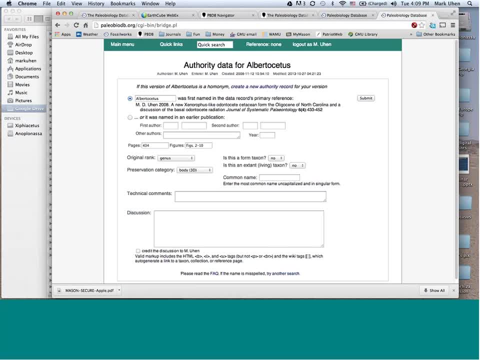 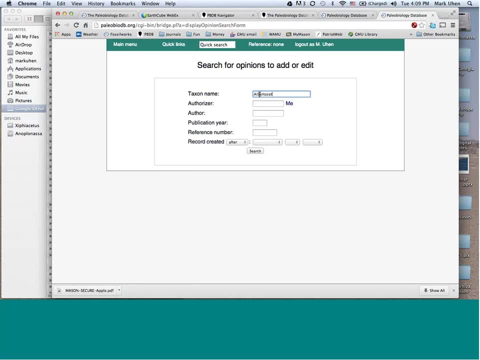 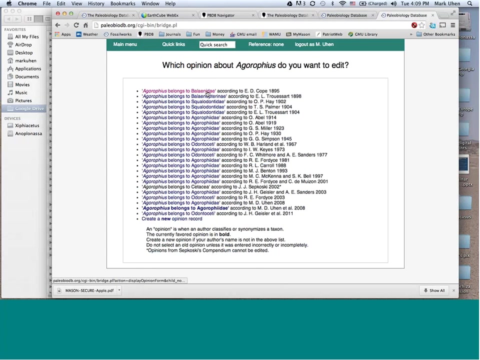 whether this was correct it is, then we can also look at opinions about those taxa like this, this one. there's only two opinions: the original and if one that came out, both assigning it to the same family. here's one that's a little more interesting. and this taxon it's been assigned through many different families by: 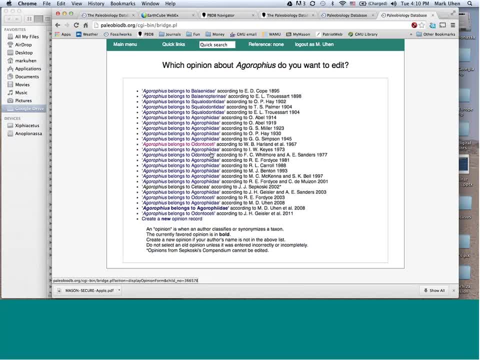 both misdeceit whales and cute whales, and then it's got its own family. but you can see all the different opinions about this one genus and how they've evolved over time, And so, in this case, the one that's in bold. 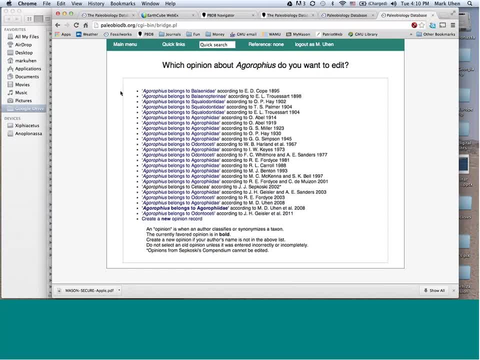 is the one that's actually being used by the database, which is usually the most recent one- not quite here, So the taxonomic information can get very complicated, but it's stored in a very rich way. You can always go back and reconstruct. 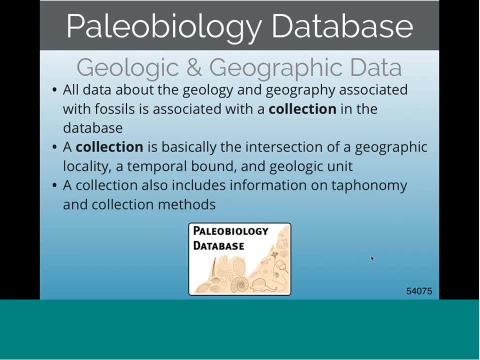 what anyone's ever said about any given taxonomic name. So the geologic and geographic data is probably the richest data type that we have, and they're all associated with what we call a collection and it's basically just the intersection of a geographic place with a temporal bound. 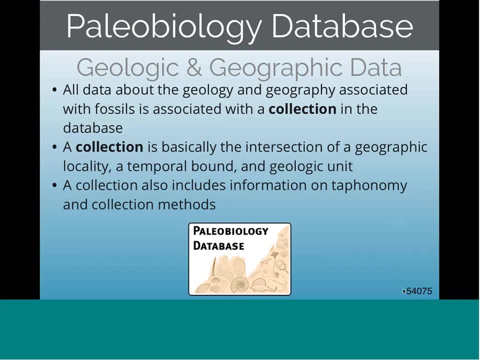 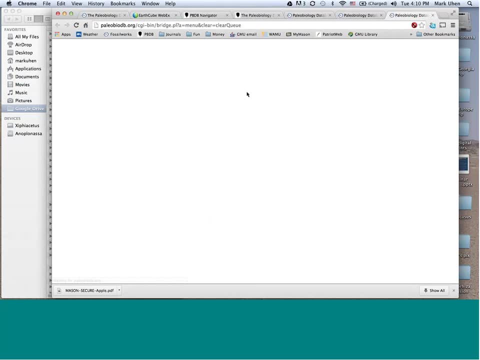 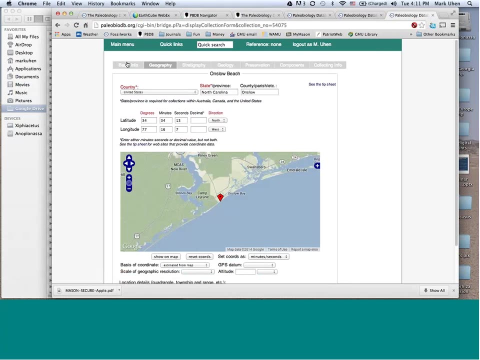 and usually a geologic unit. So we're gonna look at this collection, Which happens to be the same collection that the taxonomy we were just looking at was from. Here's just some basic info. Notice that there's multiple references associated with it. 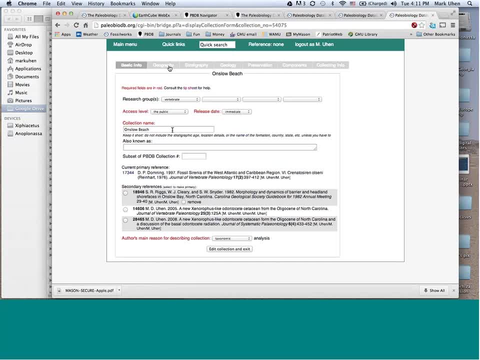 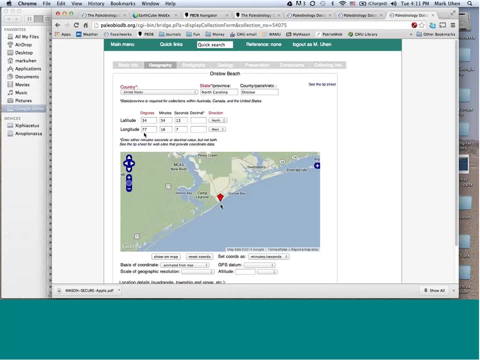 because different people have talked about fossils from just one single place. Here's the geographic info with a little map, So as you enter data you can expect to see that your dot is right where you think it should be. It's real easy to mix up your north, south, east, west. 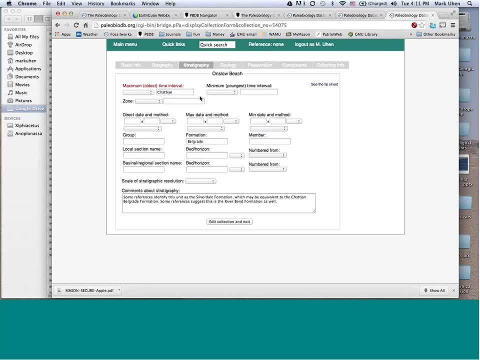 and get them across the planet. Here's our information on time and stratigraphy. We have different ways of entering time and named time intervals And there is a strict vocabulary for this. It won't let you put in units. it doesn't understand. 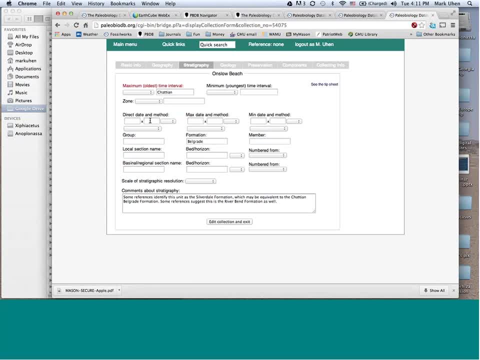 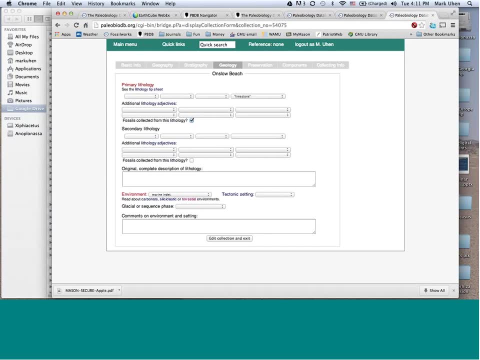 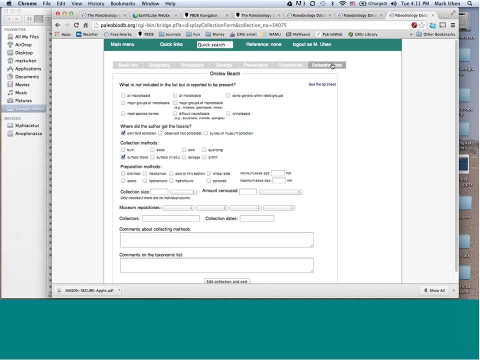 And also direct date methods to put in or direct date numbers and the methods that are used to assess them. Here's stuff about the lithology and the environmental deposition, Preservation of the fossils, What's in this collection of fossils, and then here how it was. 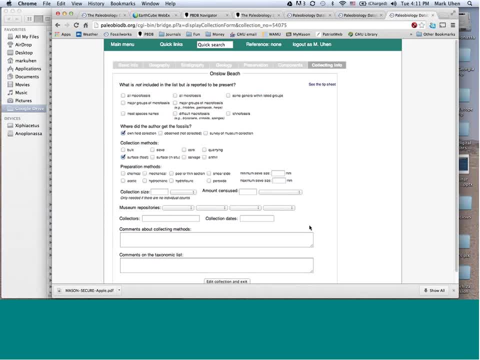 collected and even some about where the collection is stored. And most of these fields, or these groups of fields, have places to put comments, So if your data doesn't seem to fit in any particular category, you can always add it to the comments field down here. 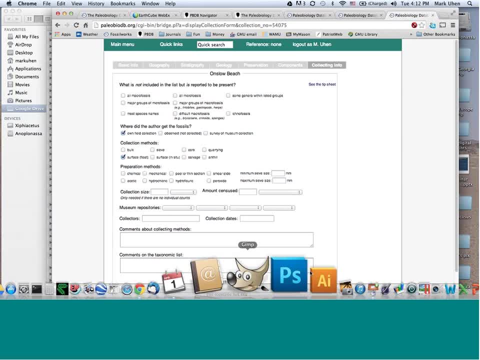 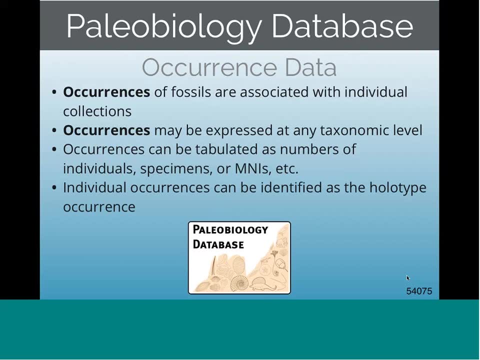 All right. our next data type are occurrence data. We'll look at the occurrences for the same collection here, And these can be expressed at any taxonomic level, down to the species or subspecies and all the way up to any higher classification that you want. 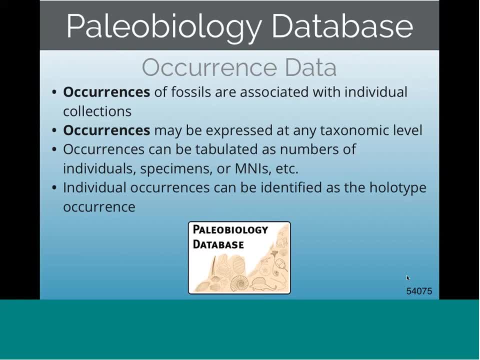 So here's the data type. Here's the data type, Here's the information that you might have, And we can keep track of them as occurrences or numbers of individuals, specimens, MNIs, all sorts of different ways to track numbers of things. 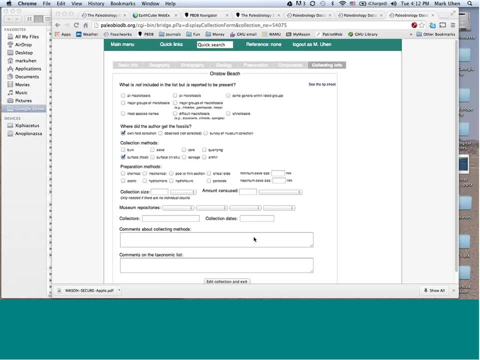 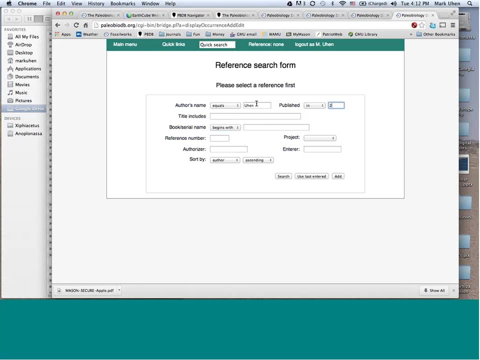 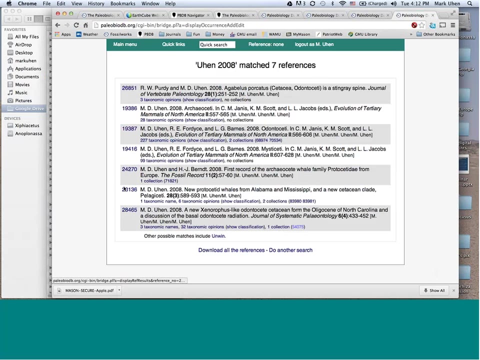 Let's go take a look at that. It won't let me do this without having a reference. I'm gonna grab one. Let's see. Here's the same collection, but now we're looking at the list of things from that place. 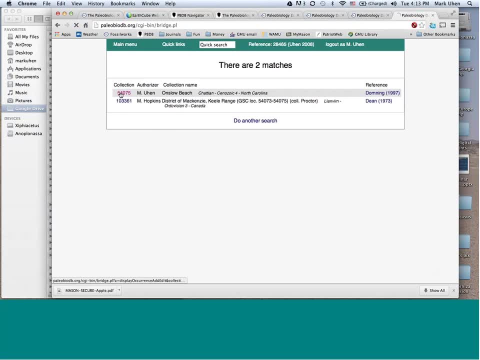 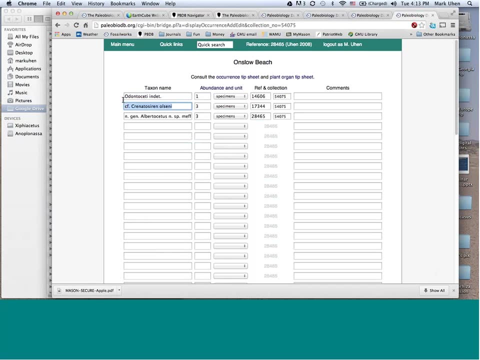 And you can see. here's some at the subordinal level. Here's a CF species, And note that- and this is where we also say that it's a new genus, a new species, So you can actually keep track of the type, locality. 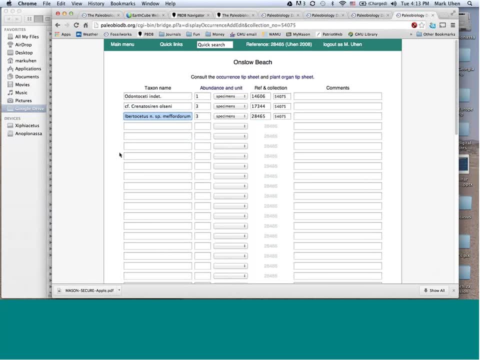 as long as it's indicated here that it's a new genus or new species That will get associated with this collection, And you can see that the subordinal is kind of a list of things that we would like to keep track of, So we can go ahead and do that. 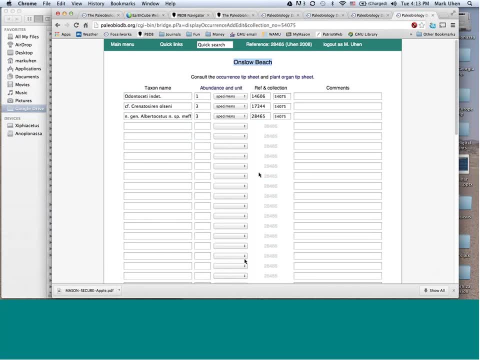 name and collection number, so you always know what, the type, locality of any given tax on you, as long as that information is entered here. now, that's how most of the data is entered and you can also explore it and retrieve it in a bunch of different ways. so all the things I just showed you actually use these. 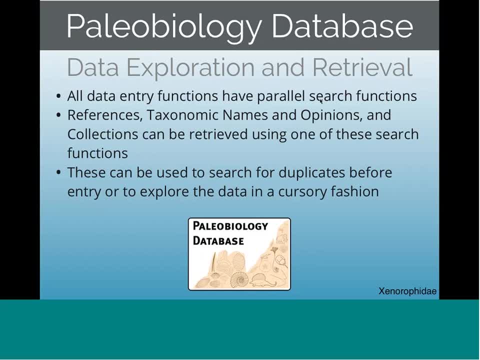 search functions to find stuff that was already in there. so we looked at the data entry screens. we actually use the search function to find them, and all all this information, all these information types, can be retrieved by using one of these search functions. so I can even go find. let's go look at all the data. 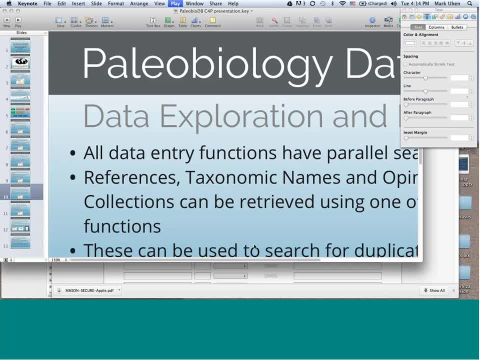 associated with this family so I can search for collections of that family. so there's the data entry screen and I can actually use the search function to find there's the one we've been looking at and notice there's a whole bunch of other collections that have fossils that have identified as members of the 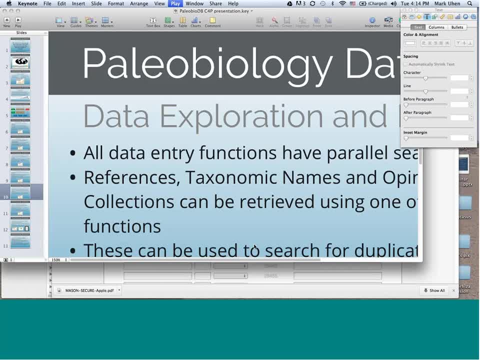 numerosity, the family, that thing. so you could go drill down and look at these. you could download this data whatever you need to do, but this is right now just a way to browse and look at the data, and you can also use these search functions to look for. 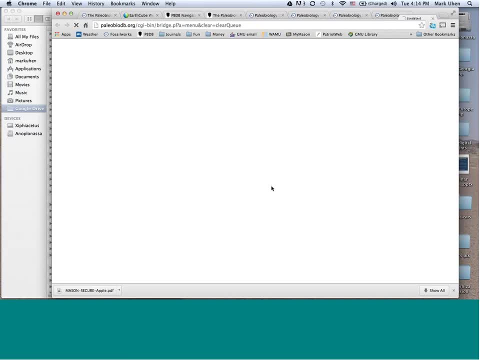 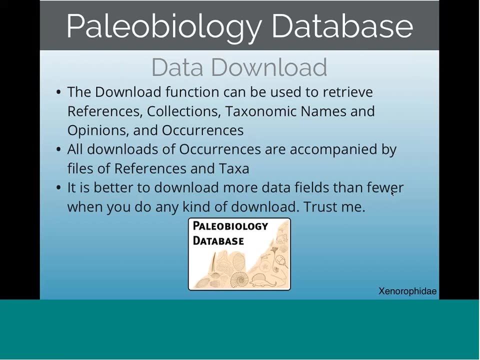 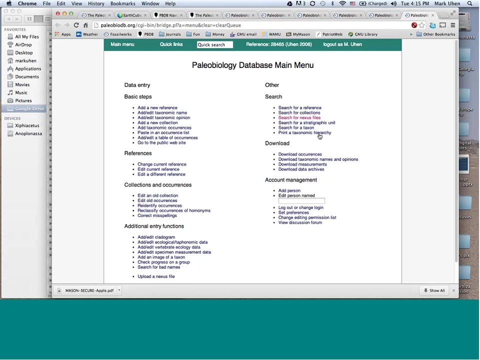 duplicates like. we don't want you to enter the same paper twice, so use those search functions to see if a paper has already been entered before you enter it again. now you can also download the data using very specific functions, so let's go download the data associated with its family right here. there's a whole bunch. 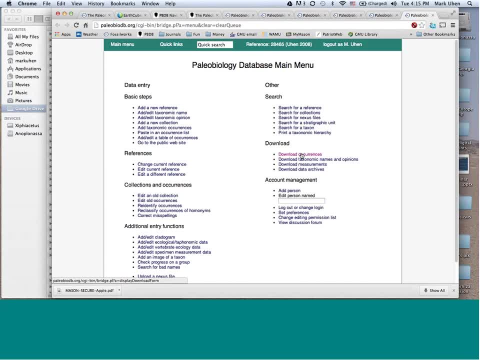 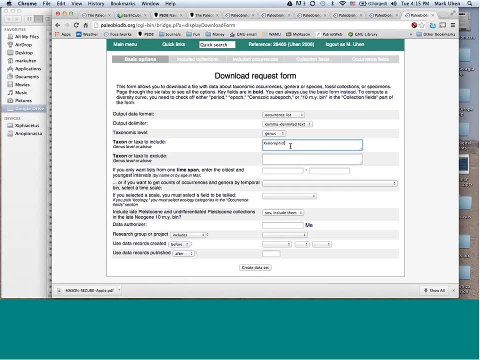 of depending what kind of data you want. hit one of these. one of these buttons over here will be the references- and notice that you can restrict the data in many ways here and you can actually include lots and lots and lots of different data that we store by going. 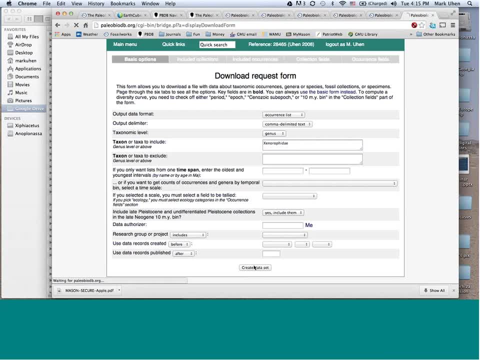 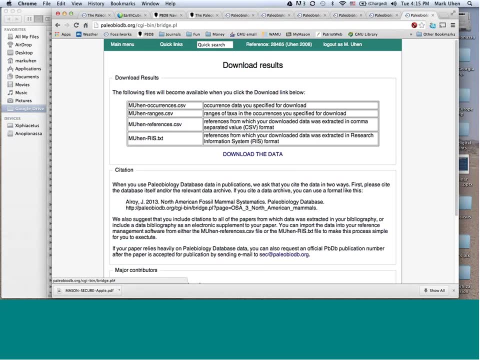 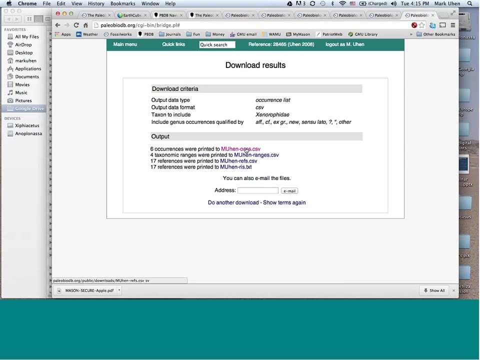 through all the fields, which I'm not going to do now for 10 seconds. but here you just hit the Create Dataset button. You're going to get a list of occurrences, ranges, references in two different formats. And here they are. So notice: it found six occurrences, four ranges with a different taxa. 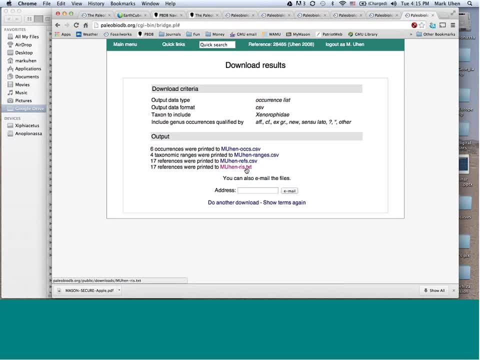 and then the references in two different formats. You can download it as RIS and put it right into your bibliographic software to make a bibliography of the data of the papers that were used to create this dataset. It can be really handy when you're at publication time. 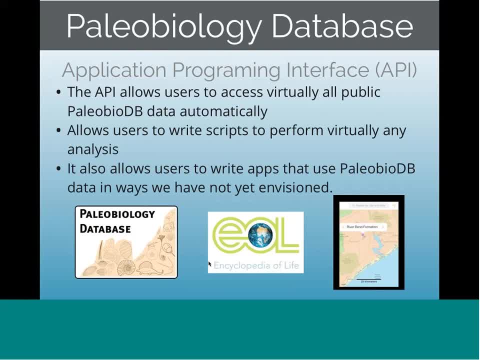 And I also want to talk just briefly about our API or Application Programming Interface, which has just recently been released, And the API allows users to access virtually all the public data automatically. You can write scripts that perform all these functions. I've been using the website for. 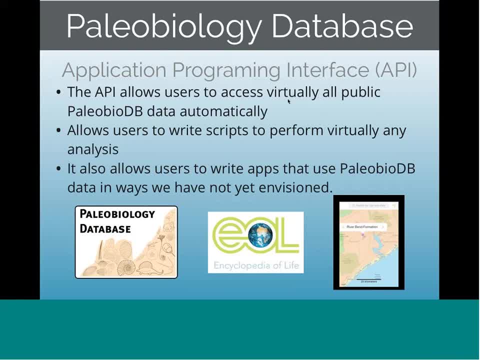 You can write a script to download the data and then perform analysis on the downloaded data, which is really useful. It's really really handy And, in fact, you can write apps that use the Paleobiology database. Like if you've never seen it, there's an iPhone app called MANCODE. 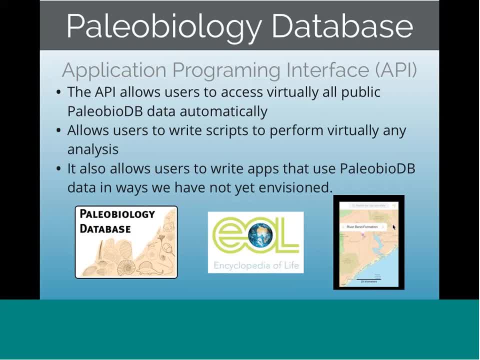 written by Steve Holland and his crew that draws in geologic data and fossil data from TBDB And you can visualize this data, along with the geology, right on your iPhone or iPad. It's pretty amazing. We have a lot of other data partners that are using our data, like Insectiology of Life. 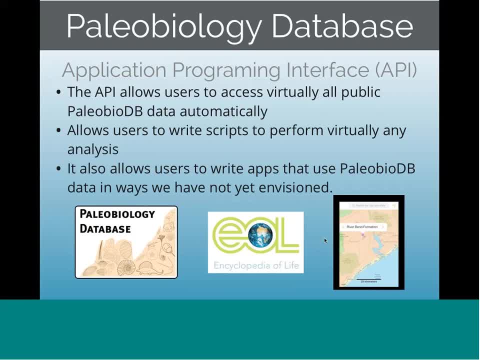 which is currently using our dynamically generated taxonomy app, And we have many others, and other people are coming on board all the time. But every single person on the planet can use this functionality as long as they know how to access the API, And this is explained on our website: how to get at the data and the protocols for doing so. 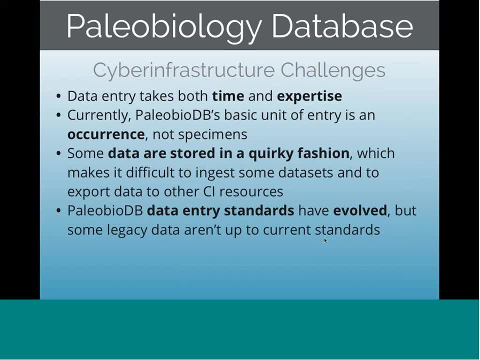 So, lastly, I just wanted to close with this sort of musing about cyber infrastructure challenges that we're experiencing right now And some thoughts about what we're doing with them. So data entry takes both time and expertise. You can't just jump into it untrained. 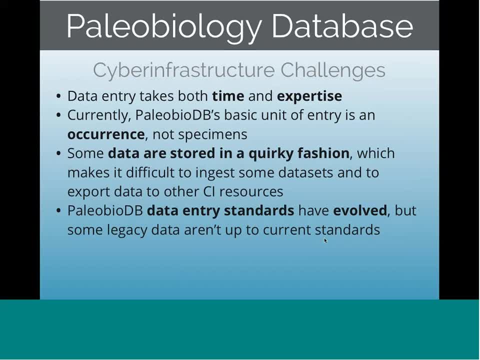 And so it can take a long time to enter a single paper if there's a lot of fossil sciences in there and a lot of taxonomic experience. So Shannon and her team on a different project has been talking about trying to automate this and having machines actually read papers and format the data for things like paleobiology data. 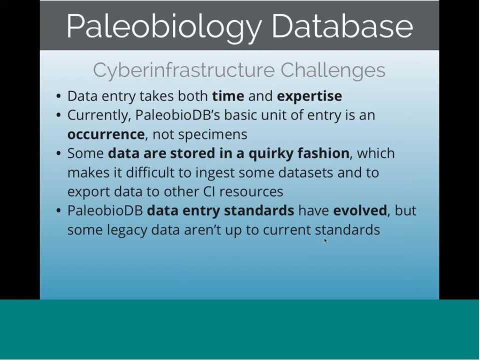 Which might be a huge leap forward for us, But right now that's in the testing phase Again. currently our unit of entry is an occurrence- We don't track individual specimens- But we're looking to expand our data input to actually take in specimen data. 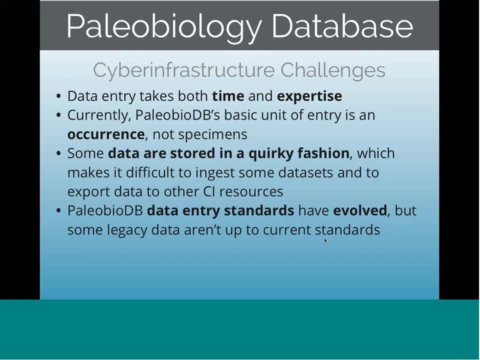 So we might be able to actually import data from museums and reformat them into the sort of way we're used to dealing with them, And some of our data- and some of our data- are stored in a quirky fashion, because our database started 12 years ago- more than that. 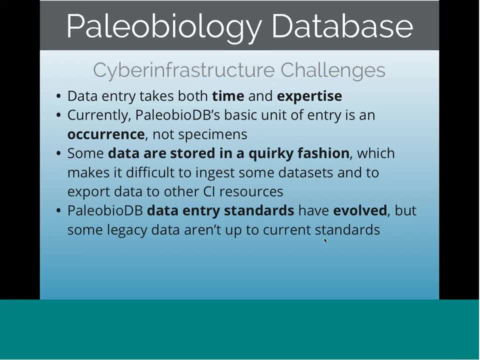 And so it was done. before. there were a lot of data entry standards, And some have been set since then and some have evolved, And PBDB has certainly evolved with it. But some of our old legacy data aren't up to standard, And so we're trying to standardize how we store and exchange data. 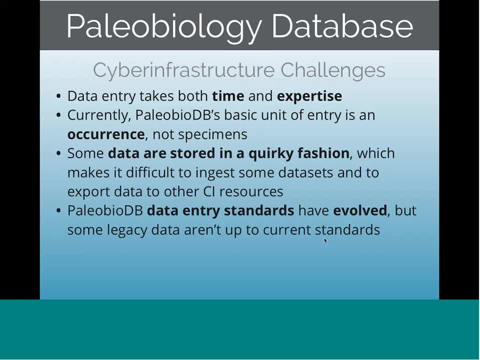 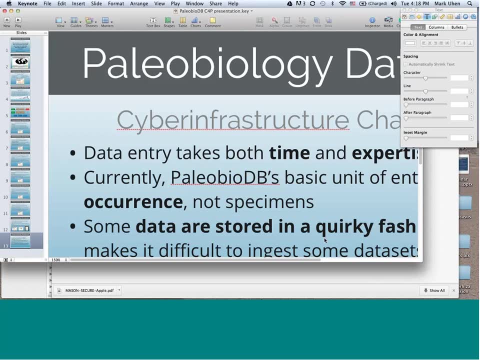 to make it more useful to people who want to draw it in using our API for whatever purpose they want to use it for, And I've ended a couple minutes early. I can certainly go on and on, But I'd rather open it up for questions and let you guys ask me whatever you like. 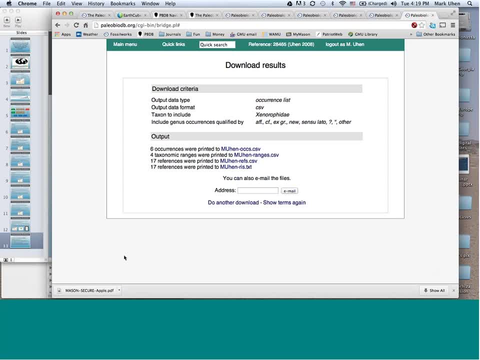 And hopefully I can show you what you need to know about either using the database or becoming a member. And if you want to actually enter data, I should say that the easiest thing to do is just email info at paleobiodborg and send us your CV and what you want to do. 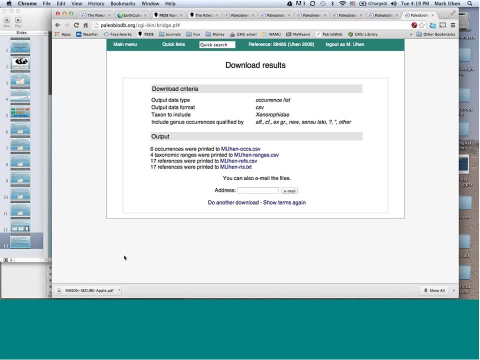 and we'll pick it up. Thank you very much, Mark. Again, if you have questions, please go ahead and type them into the chat window and Leslie will collect those and present them to Mark here. Leslie, do we have anything to start with? 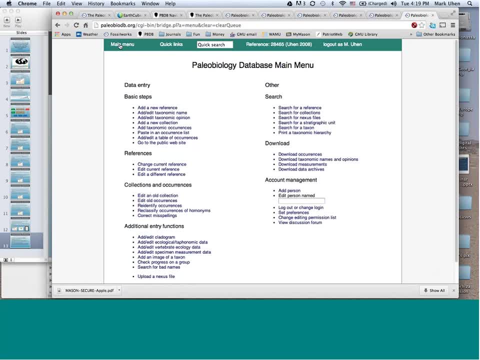 Yes, we do. The first question is: what timeframe do you anticipate folding in specimen data related to literature, references and other things? We don't have a timeframe yet And we do take in some kind of specimen data, but we don't use it to construct the current list. 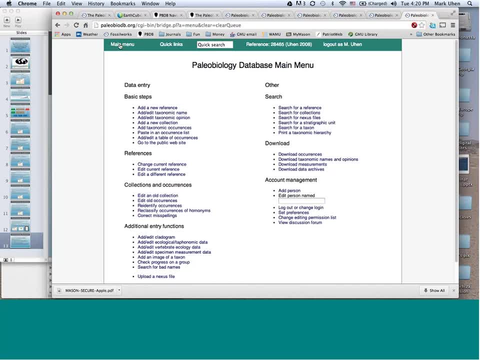 So, yeah, it's going to be a little bit- at least a year, I would say- before we're ready to do that, But we're exploring options right now and also exploring using some of the more global universal specimen identifiers as well. 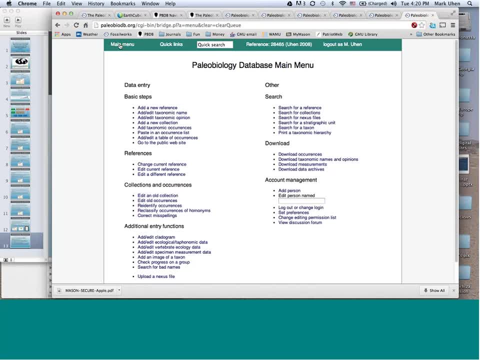 so that specimens will be able to be tracked both within our database and other people's databases using the same specimen identifiers. So hopefully that will make it much more easy to exchange data among different systems. All right, thanks. The next question is: what are your main channels of user feedback? 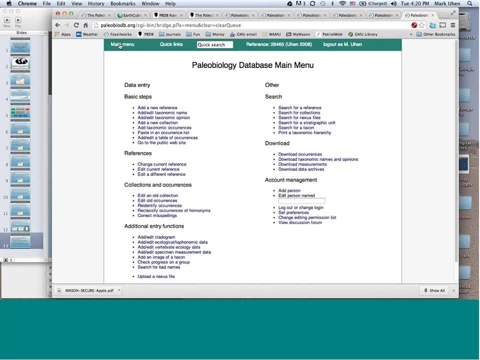 and how do you prioritize? That's a good question. Usually just via email and conversations with people. So people we set up this info at paleobiodborg email to send general questions to, and that goes to me or Jocelyn Cessa, our secretary. 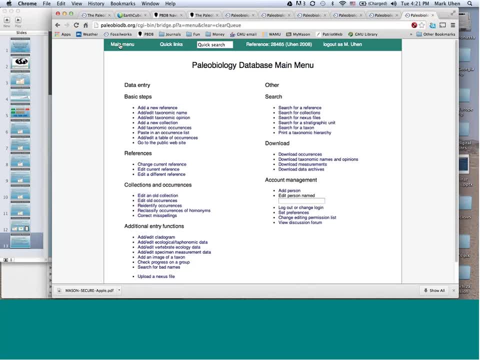 who we're pretty good about either answering them or sending them off to other executive team members or our IT team, if they're technical in nature, and trying to get them answered right away. If there's a bug that can be addressed very quickly, we try to do that. 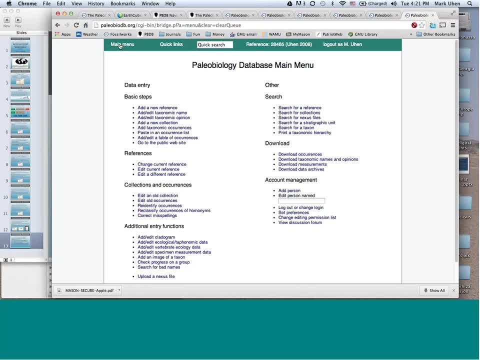 But if not, it either goes on our troublesome bug list or our feature request list, And both of them are pretty long and we have basically two half-people programmers working on them. So we do our best And for the most part, 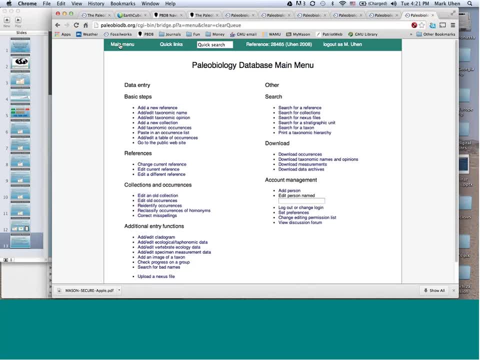 what we have works pretty darn well, But we're always looking for new suggestions for people, Even if they don't come out right away. they're going on our list. Okay, I had a request to read the questions louder. Hopefully this is better. 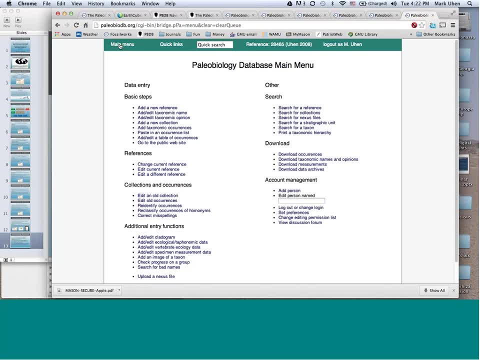 The next question is a little bit related. When an error is found in the database, who is best to alert the error, the authorizer or the info at email? The author or authorizer? Yeah, So every record is attached to the person who entered it. 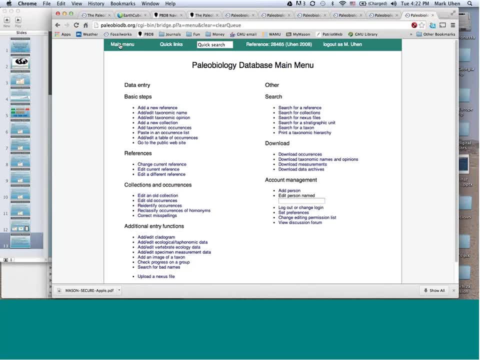 And that's the person we call the authorizer, And it's best to email them directly because they're the people best to fix any errors. If you send it to info and that comes on my desk, I'm just going to turn it around and send it to authorizer. 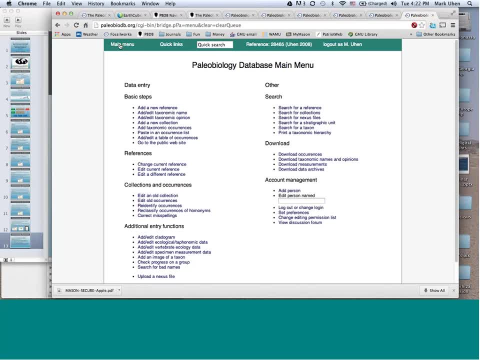 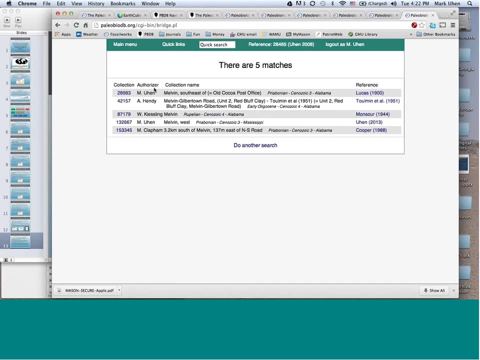 So that's your best option. Your best bet is to go directly to them And so you can see their names associated with the record, like here. Let me find one. So here, this record for Melvin is associated with you, So you can find a list of everyone in the database. 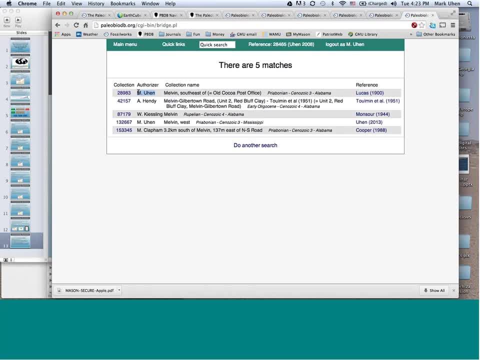 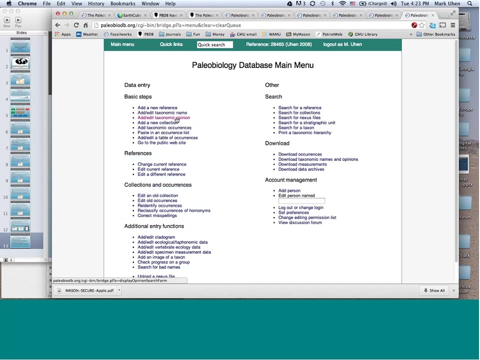 in our info pages and you can find their email and send it right to them and hopefully they can help you out. Okay, great. Next For the taxonomic opinions. who maintains it? Is it mostly the authors themselves, or are there some authorizers who do most of the work? 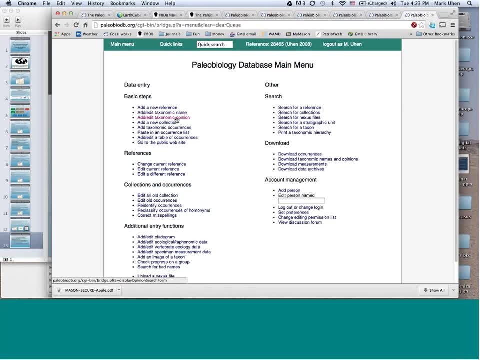 putting this information in. The only people that enter data are authorizers, So the authors themselves, unless they are authorizers, aren't doing that, And this is sort of a different feature of the database. A lot of systems have a single hierarchy. 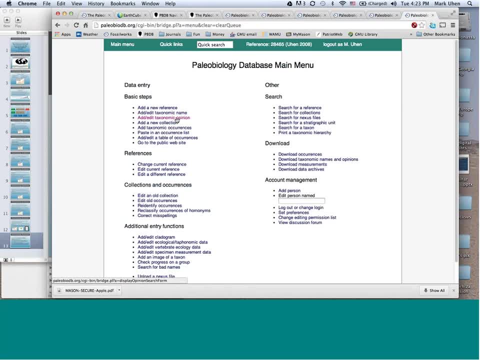 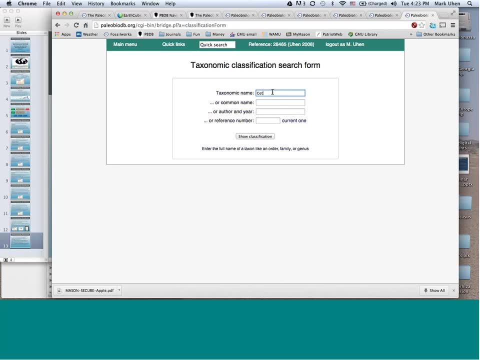 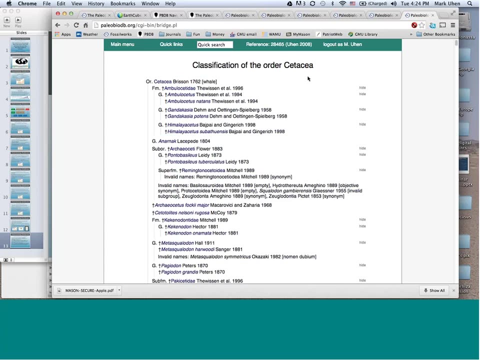 taxonomic hierarchy, sort of enclosed on the data, where ours is actually dynamically generated. So let me show you what that means. Since I work on whales, let's look at whales. So here's this. This is a classification of cetacea that it just generated for me on the fly. 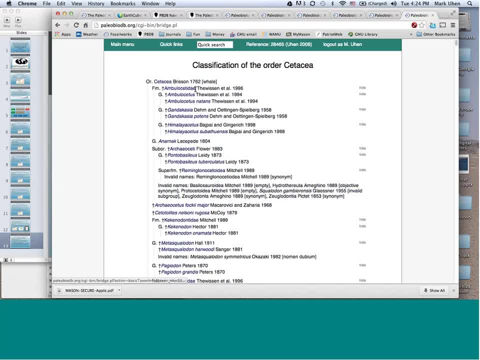 So there are opinions saying Ambulocetis belongs to Ambulocetidae. I didn't tell it that. There's a series of opinions that say that, And so nobody maintains the hierarchy. It just generates itself based on the most preferred opinions. 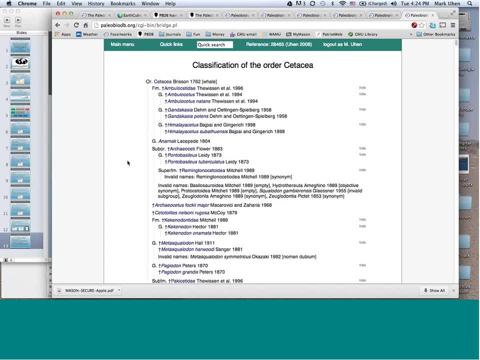 that have been entered, And so sometimes we get a lot of- I get a lot- of emails from people saying, oh, I don't like the way this taxonomy looks, and the only answer I have is: if you don't like it. 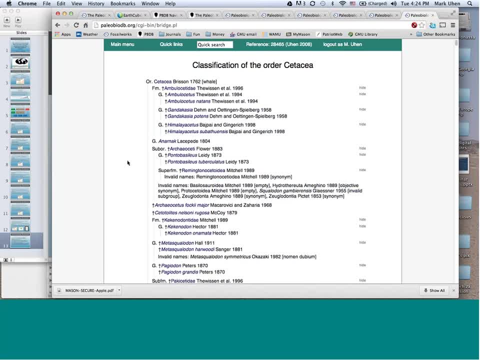 jump in and enter some more data, because that's the only way to make it look any different. Okay, the next question is: how did you encourage participation to get the database where it is today, with the amount of data that's in it? 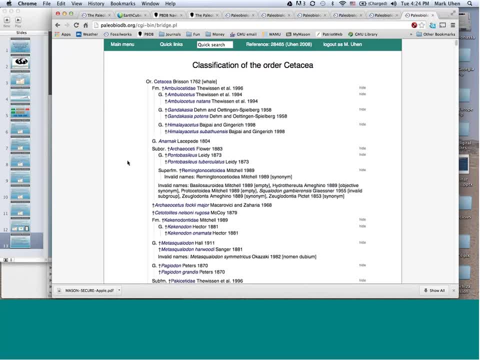 That's a really good question And I'll tell you my own personal, my own personal reason for entering this data. I've entered all the marine mammals and all the marine birds and all sorts of stuff, And I did it for my own personal, selfish reasons. 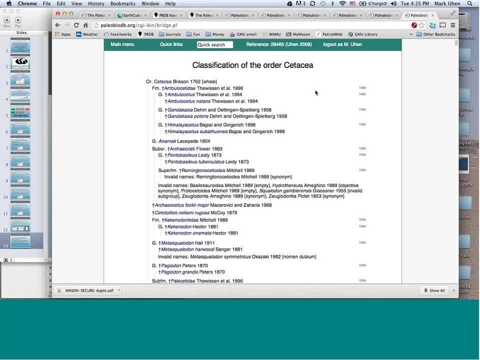 I wanted this data in here so I could re-extract it and do interesting science on it. And I figured: why shouldn't other people benefit from my time doing the data entry, You know, rather than just put it into a big Excel spreadsheet? 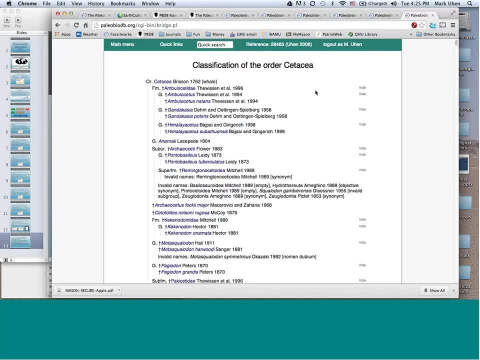 or some personal database. this way it's out there, it's available everywhere the web is and everyone else on the planet can use it. So I think there's as much science that was done on the data I've entered by other people than me. 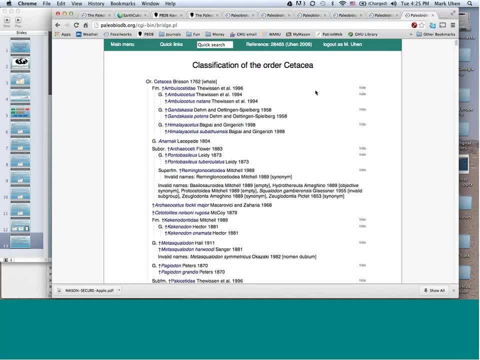 And so I encourage people to enter data for their own selfish reasons, and then you get the data that you want to use, And yet there's a lot of added benefit by letting other people use it in ways that you never would have thought of. 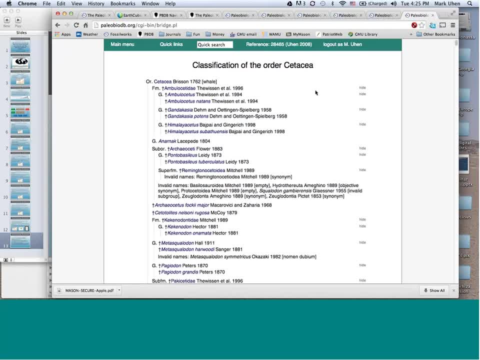 Or you could generate new collaborations with people who want to use your data in ways that you might not have thought of either. So I think, join for selfish reasons, oops, but then you get this extra benefit of being a public resource, And I think that's true of most people. 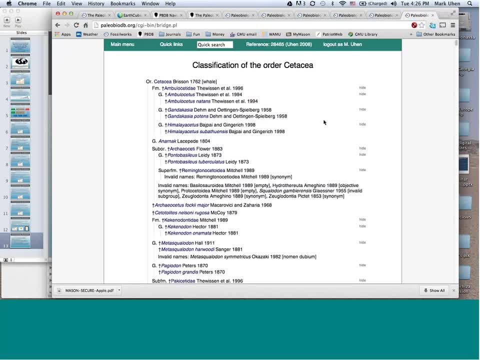 who are in the database, and this is how we got most of this data. Okay, next question is: are there plans to allow for the batch upload of collection data, Perhaps a digital form that would streamline and minimize data entry error, The data entry process? 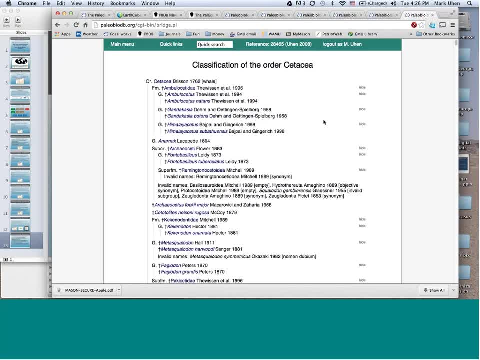 for non-standardized collections, for example, collections currently housed at the Smithsonian. Yes, so that's what I said before about: we're looking to enter specimen data That falls under that category. So, yes, that is our the next great frontier for us. 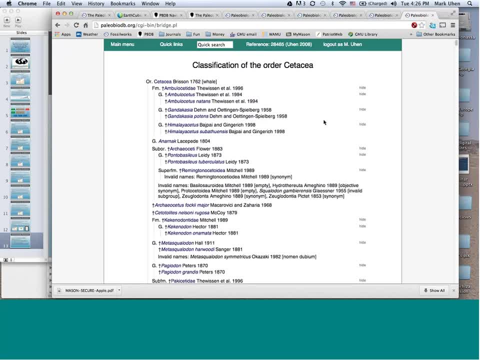 is getting that in And we're talking with a couple of different groups that have specimen data about how best to do that. So, like I said, it's kind of a big task. So we hear you. We've heard this from a lot of people. 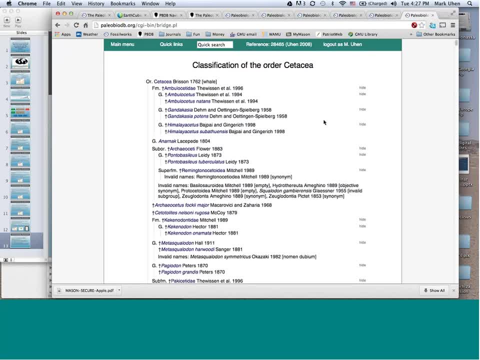 and we're definitely moving in this direction, but it's gonna be a little bit until we're ready for prime time with that. Okay, that's the last question right now. Nothing else is showing up right now. Okay, Great, So actually. 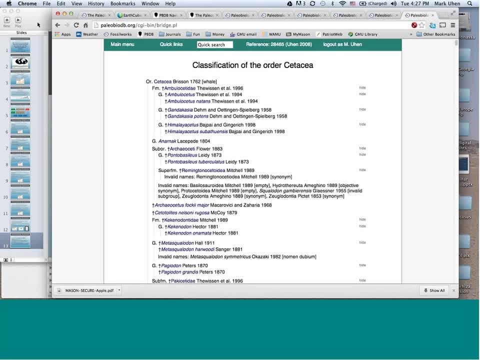 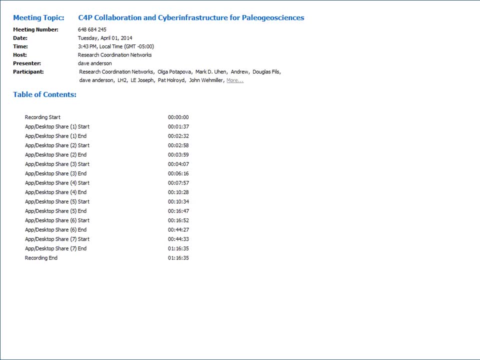 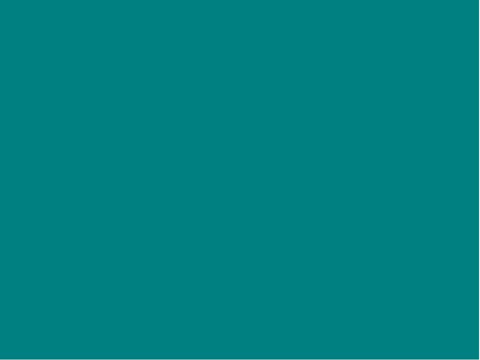 the timing's about perfect, So we'll go ahead and move on to the next presenter, Dave Anderson, on the World Data Center for Paleoclimatology. So we'll pass the ball to you, Dave Great, How are we doing, Josh? 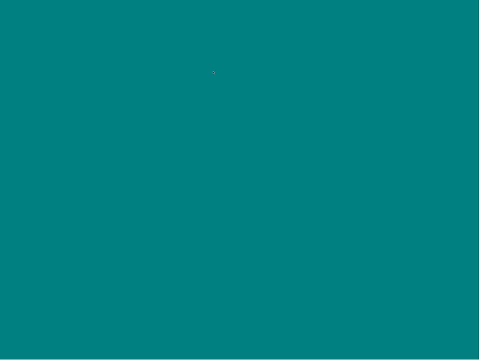 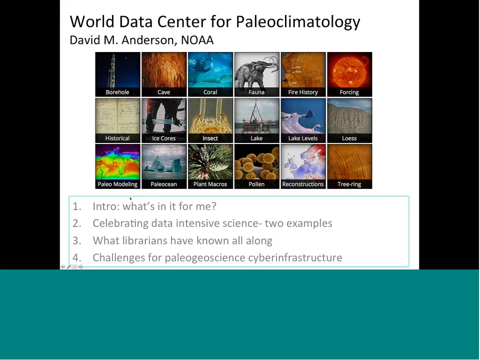 Let's do a sound check. Is my voice okay? Yes, You're doing fine, Great, And can you see a screen labeled World Data Center for Paleoclimatology? I see that and I see you. Good, Good afternoon everybody. 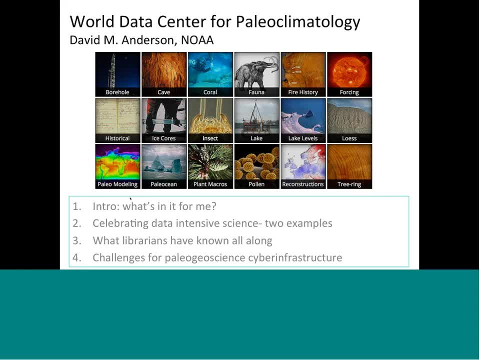 My name is David Anderson. I'm the director for the World Data Center for Paleoclimatology at NOAA's World Data Center for Paleoclimatology, And I'm here to talk to you today about the world data center for paleoclimatology. 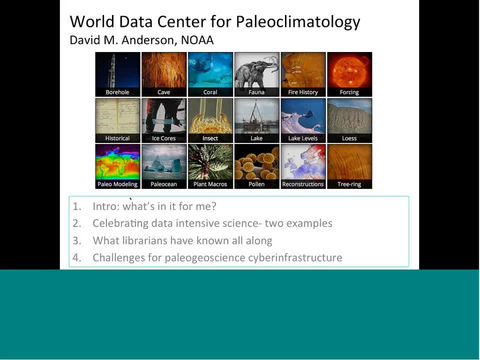 I'm David Anderson. I'm the director for the World Data Center for Paleoclimatology at NOAA's World Data Center for Paleoclimatology at the International Climatic Data Center in Asheville, North Carolina. This webinar is part of the Research Coordination Network. 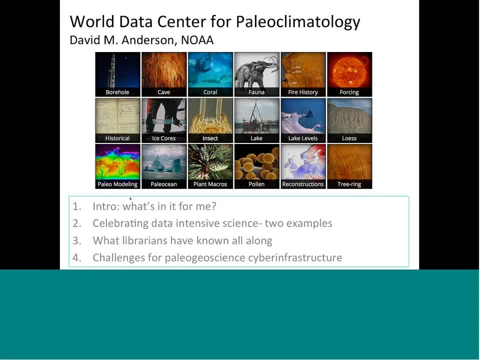 for Paleogeosciences webinar series, And I'm really excited to be able to talk to you today about the archive at NOAA, which consists of paleoclimate data submitted and, you know, contributed by scientists working at institutions around the world, based on their 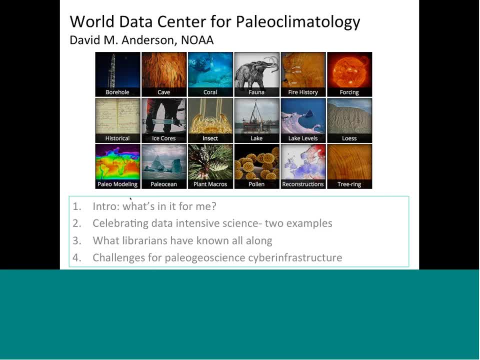 published research using some of the proxy types I'll find here. So in this talk this afternoon, I'm going to first begin by answering a question for you- What's in it for me? And I'm going to try to describe some of the things. 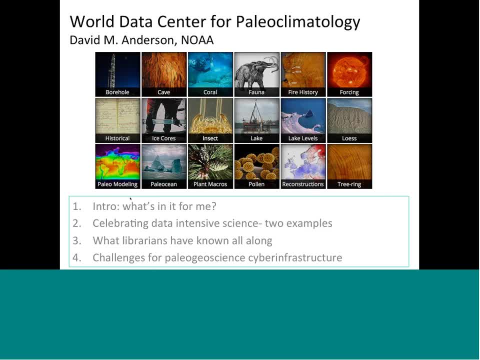 in this archive that you might find of interest in your own studies and research and data efforts. And then, for a moment, we're going to celebrate data-intensive science. I'm going to tell you some stories about scientific discoveries that have been made possible. 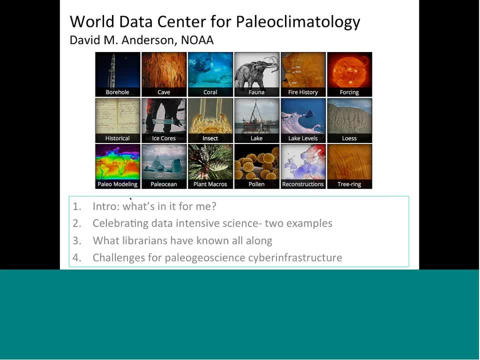 by data-intensive science, discoveries that would not have been possible without the archive efforts that we're talking about today- And you know, at the end of the day, that's really what it's all about- is enabling data-intensive science through the development. 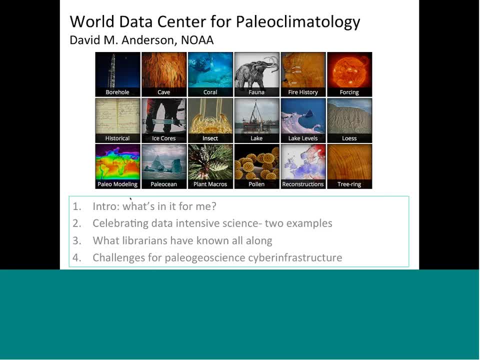 and the connection of these different archives and different tools. So then I'll tell you what librarians have known all along, and then I'm going to talk a little bit more about data-intensive science and how data-intensive science can be used for the. 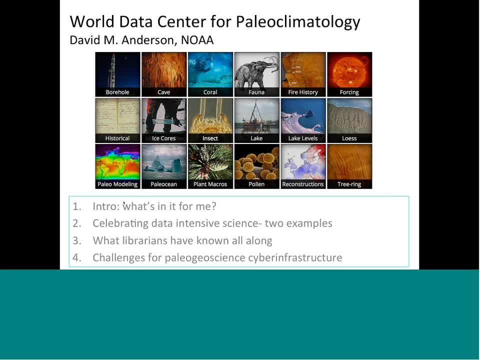 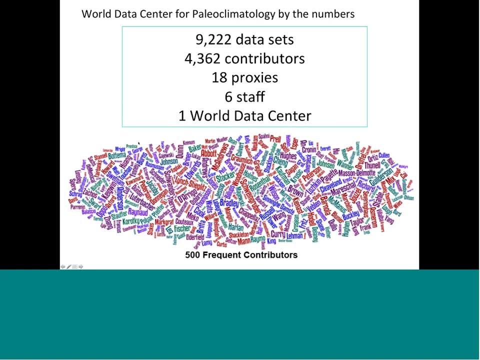 paleo-geosciences- cyber-infrastructure in the last part of my talk. Doug, I am having trouble advancing my screen. Oh, there we go. Okay, So let's look at the World Data Center for Paleo-Climate Biology by the numbers. 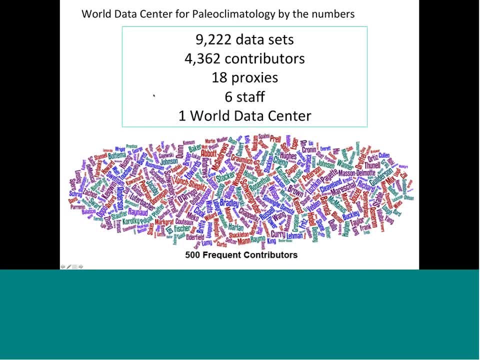 There are 222 different data sets as of yesterday. These have been contributed by 4,362 contributors working at institutions around the world. The paleo-climate community tends to organize or be discipline-specific. We call these disciplines proxies, For example. 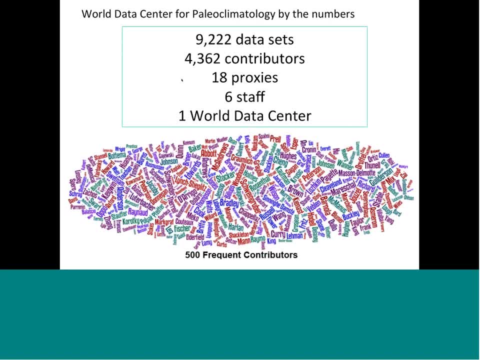 many of the journals are discipline-specific, such as the journal Paleo-Gymnography, and we recognize 18 different proxy types. The World Data Center is maintained by a staff of six people that operate one World Data Center for NOAA. The archive contains some of the most. 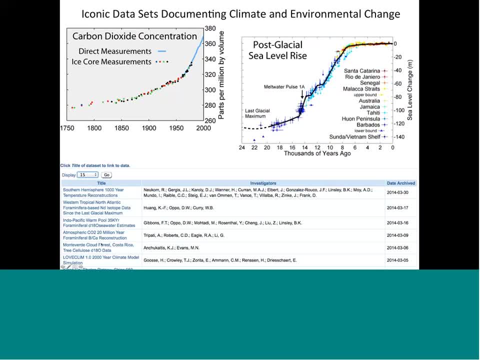 iconic and well-known data sets documenting climate and environmental change going back over the last several centuries to millions of years. And in the upper left here you can see the concentration of carbon dioxide measured in ice cores going back over the last several centuries. So this shows. 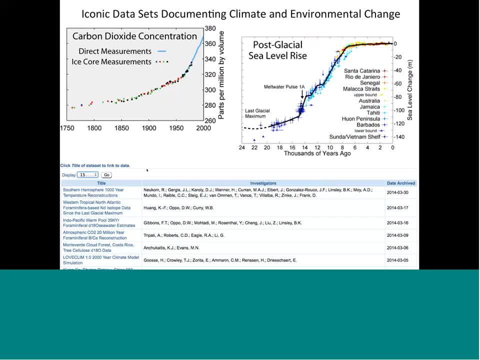 the concentration of carbon dioxide in the clean industrial atmosphere as measured by bubbles in ice core, And on the right you can see the data sets bearing on the or revealing the rise in sea level that occurred at the end of the last ice age 21,000 years ago. 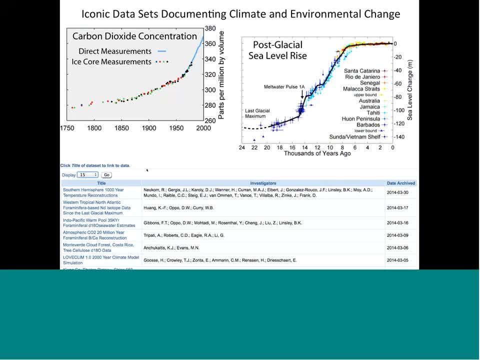 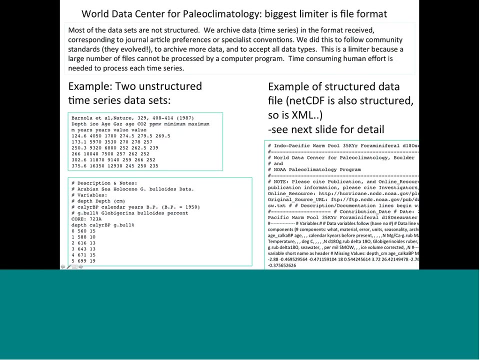 These data come from all over the world. As I mentioned, they come from all over the world And the list at the bottom shows the last half a dozen contributions that have been received over the past several weeks at the World Data Center. One of the 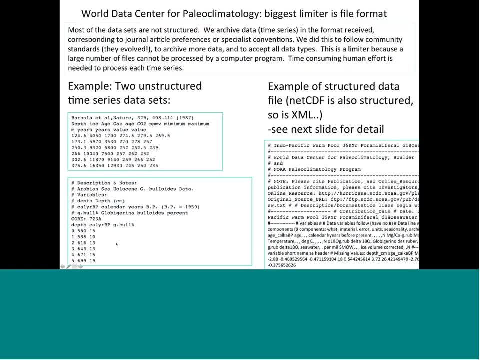 biggest problems or limiters in this archive is the file format. We've been in existence in 1991 and over that time we've collected an archive data set on the lower left of this screen that are in slightly different formats, So all of the information. 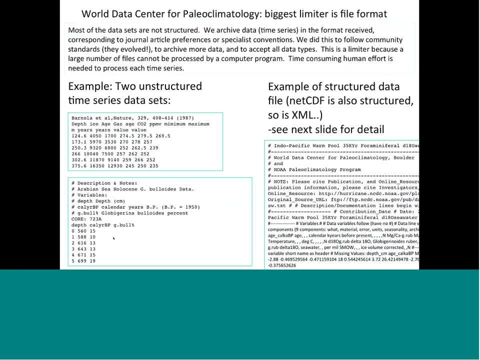 you need is there: Sample, depth, age, the variable measurements, And if you wanted just one of these data sets, it would be fairly easy to just copy and paste it into Excel or write a MATLAB script to read this data. But if you wanted just, 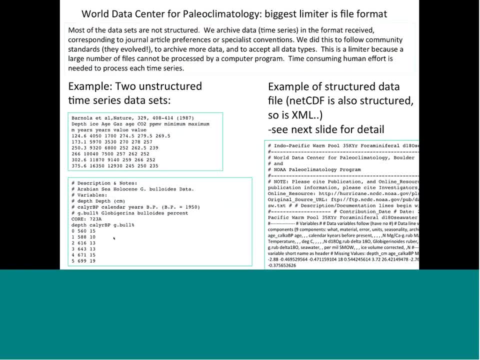 one of these data sets, it would be fairly easy to just copy and paste it into Excel or write a MATLAB script to read this data. So we archived data primarily in the format received corresponding to journal article preferences or specialist conventions. We did this in order to 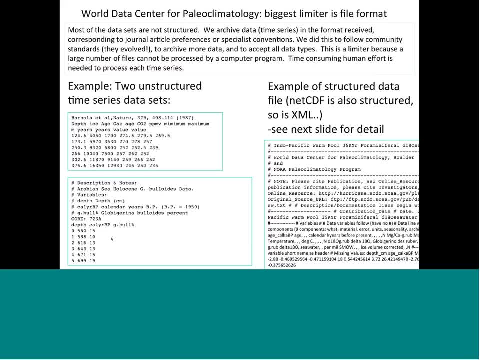 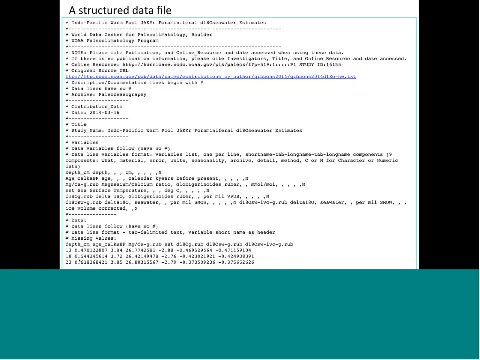 follow community standards and to make sure that we were able to meet the needs of the data that we received. So the next slide is an example of a structured data file. So in October 2013, about a half a year ago, we began an effort. 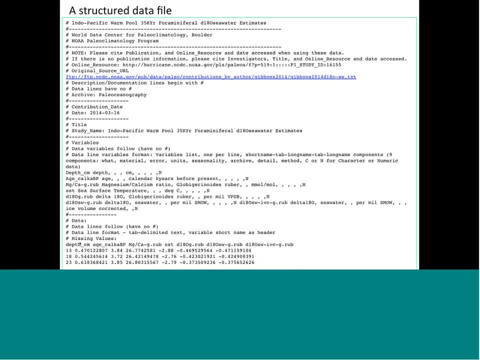 to identify the most important data that we could use in this format. So what we've been doing is structuring the data in ASCII format, where the metadata are space separated values, So formatted in this way, with an expected series of nine elements here for each variable. 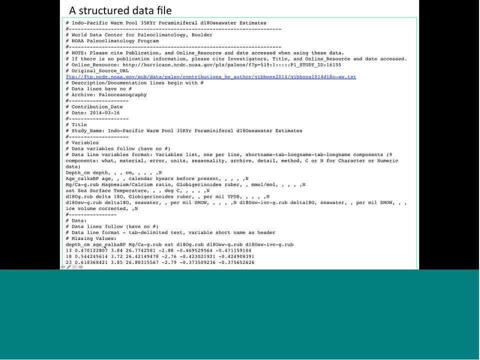 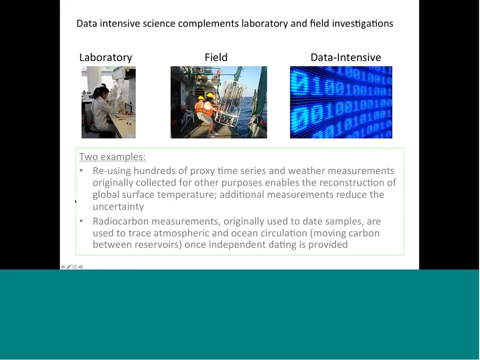 and then the data separated by spaces at the bottom. here it is possible to read one or ten or a hundred or a thousand of these files and then enable data. to the extent that we can structure the data in this big archive, we enable data intensive science. 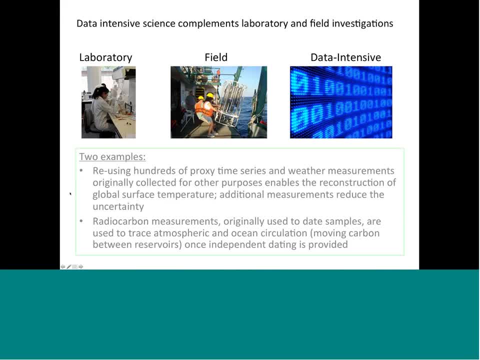 So in the next part of my talk here, I'm going to talk a little bit about data intensive, and the examples I want to show you are examples where scientific discoveries have been made that would not have otherwise been possible without a data intensive or without an archive. 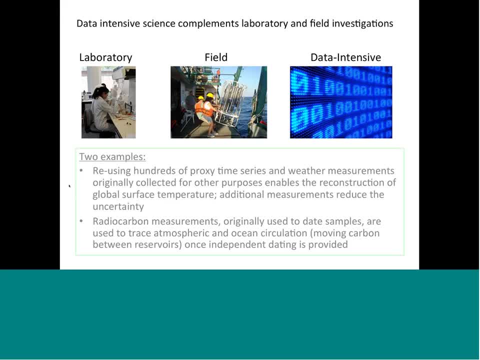 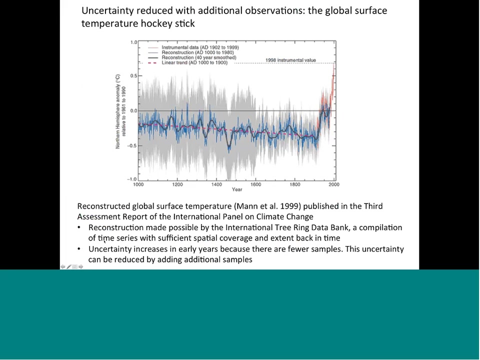 effort. So I'll describe how additional measurements can be used to reduce the uncertainty in these temperature reconstructions. And the second example I'll describe is the case where radiocarbon measurements originally used to date samples, are now used to trace the temperature of the. 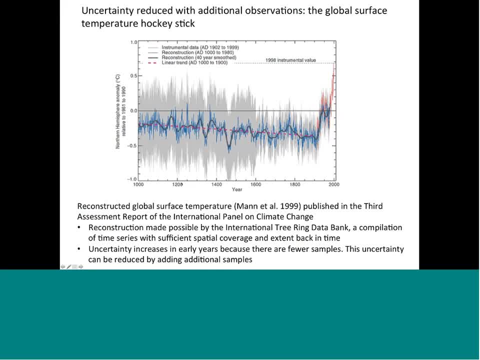 hockey stick. This is the time series of global temperature here and the interval from the present going back to 1,000 AD. The red show, the recent thermometer, shows the temperature of the hockey stick over the last 100 years and contrasting with this. 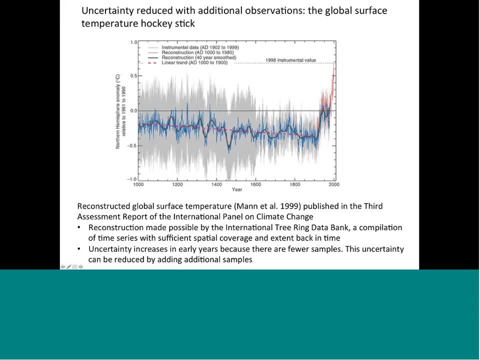 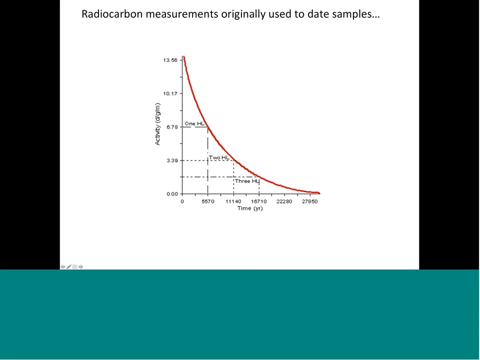 gradual cooling trend that's occurred over the last 1,000 years. These reconstructions were made possible without an archive and these data were not initially collected to reconstruct earth temperature. The uncertainty is indicated by the gray bars here and you can see how the 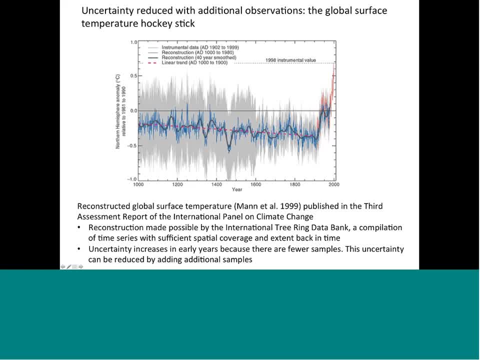 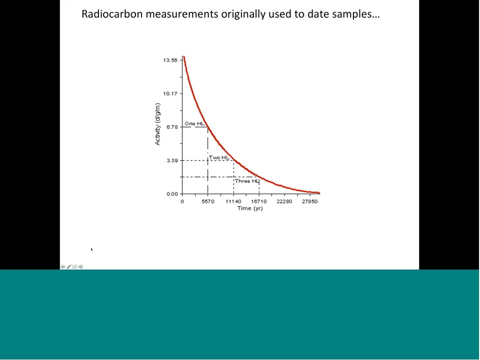 envelope of. the red shows the temperature of the hockey stick over the last 1,000 AD. The red shows the temperature of the hockey stick over the last 1,000 AD. The red shows the temperature of the hockey stick over the. 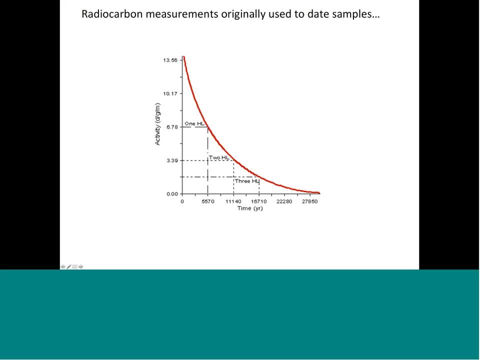 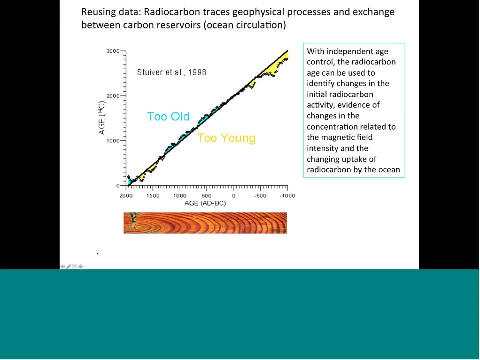 last one minute. By measuring the activity of radiopart in a geologic sample, we can use that remaining activity to understand the sample age. here What's exciting is that with independent age control we can. So the age is determined by the ring rule and the age is also determined by the radiocarbon. 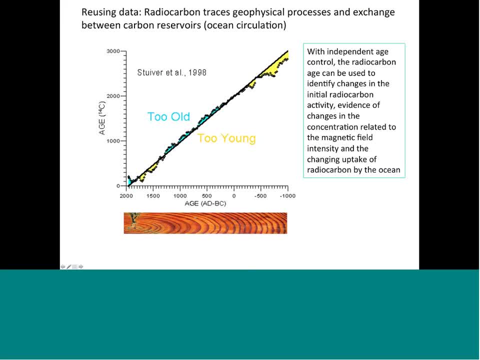 measurement And you can see here in this correspondence there are time intervals that are either too old or too young. These are times when the initial activity of radiocarbon in the sample was either a little more or a little less than this long-term average. 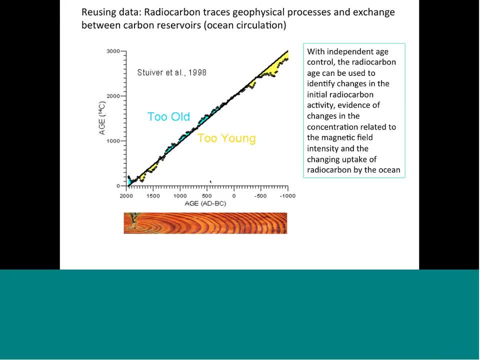 So with this independent age control, the radiocarbon age can be used to identify changes in the initial radiocarbon activity. This provides evidence of changes in the concentration related to the magnetic field variation and related to the changing uptake of radiocarbon between the ocean and the atmospheric reservoir. 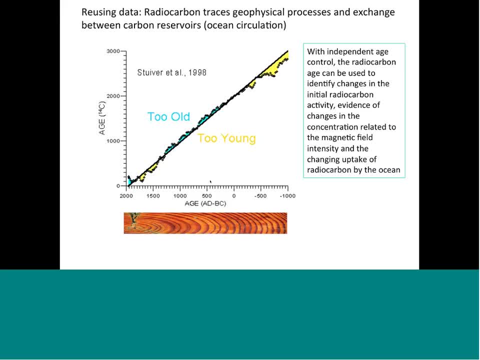 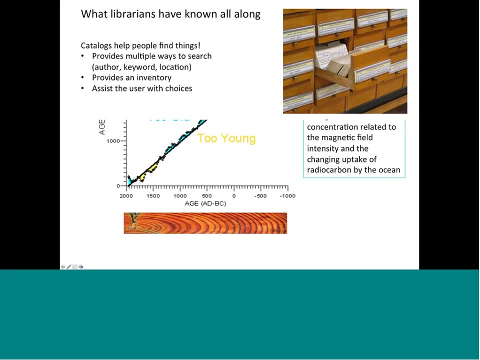 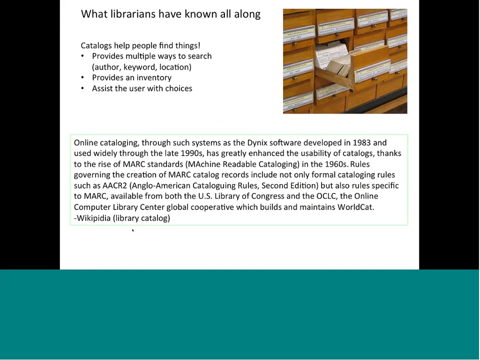 So this is another case where data originally collected for one purpose have been reused to make new scientific discoveries that would have not been possible without this data-intensive effort. So now I want to talk about something that librarians have known all along, and that is that catalogs help people find things. 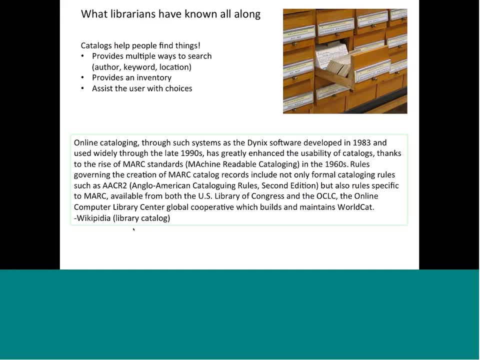 Catalogs provide multiple ways to search: by author, by keyword, by location. Catalogs provide an inventory. Catalogs assist the user with choices And I want to read to you here this description of online cataloging from Wikipedia, Because the author of this paragraph understood the power and the helpfulness of setting rules. 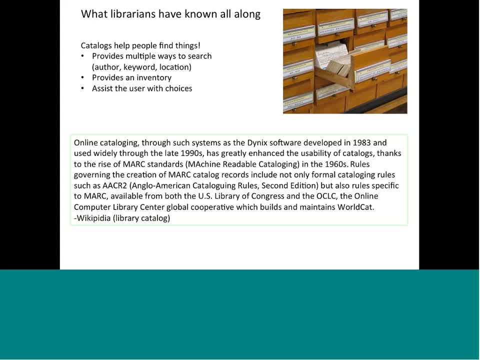 and making agreements between different organizations in the development of this catalog. So online cataloging through such systems as Dynix software, Vulkan 83,, used widely throughout the 1990s, has greatly enhanced the usability of catalogs, thanks to the rise. 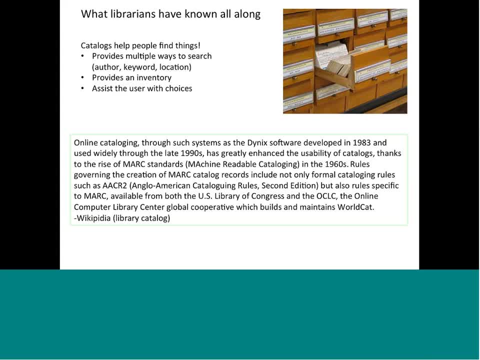 of MARC standards- machine-readable cataloging in the 1960s. Rules have changed. They have changed Rules governing the creation of MARC. catalog records include not only formal cataloging rules but also rules specific to MARC, available from both the US Library of Congress and 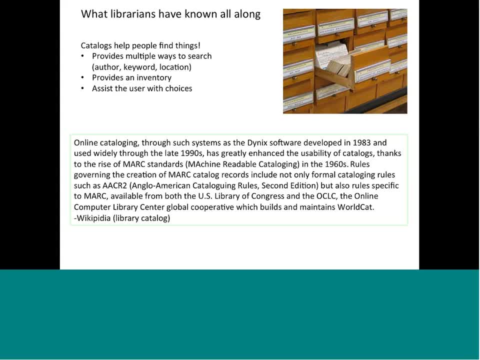 the online computer library center, Global Cooperative, which builds and maintains WorldCat. So there's a parallel here, or a moral for us in paleogeosciences, that the online cataloging that is so successfully used by library systems. So what is this about? 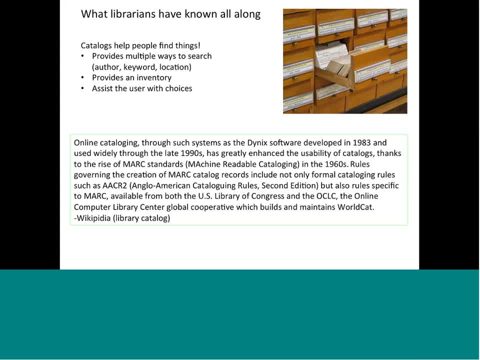 We've got some opportunities. We're not really talking about just an appearance. We're talking to people who are playing the game and we want to get that out there, And we're talking to the public. So we're talking about the framework. 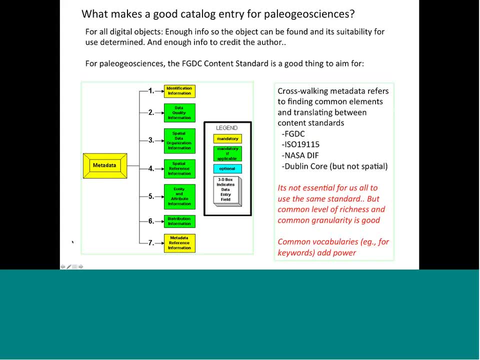 So how do we build our own interoperable catalog? So in this video I just want to talk a little bit about what makes a good catalog entry for paleogeosciences. This is kind of down into the detail. It's the technical part of our talk where we look at some suggestions, kind of what's. 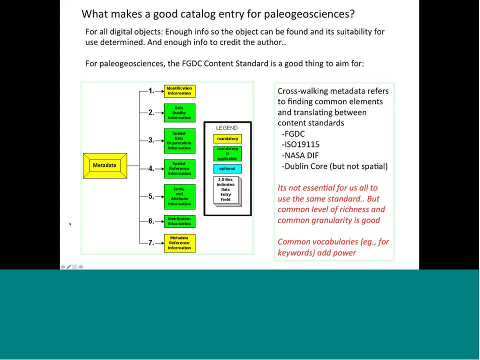 worked for us in archiving paleo data. So what makes a good catalog entry for paleogeosciences? So one of the ways it has worked for us is by looking at reviews on all digital objects. So what makes a good catalog entry for paleogeosciences? 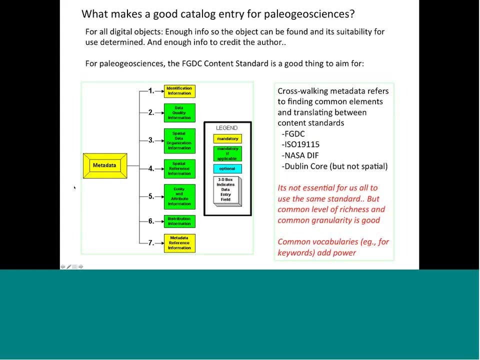 all digital objects. there's a sturdy definition, enough information so that the object can be found and its suitability for use, the common and I would add that catalog entries should also have enough information to credit the author successfully. for the paleo geosciences, where many of the data sets 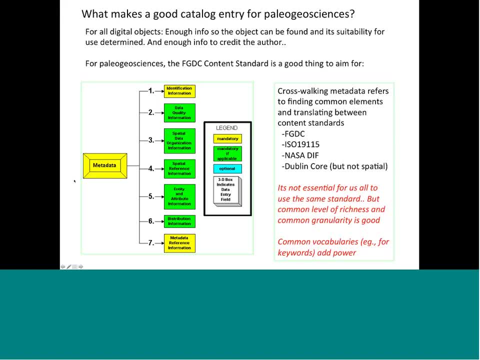 are geospatially referenced. in other words, they refer to samples that have a lot of belongs to the FGDC. content standard is a good thing to aim for and I just want to draw your attention here to the FGDC standards for meta-datas- seven elements. there is an element for identification, information- an element. 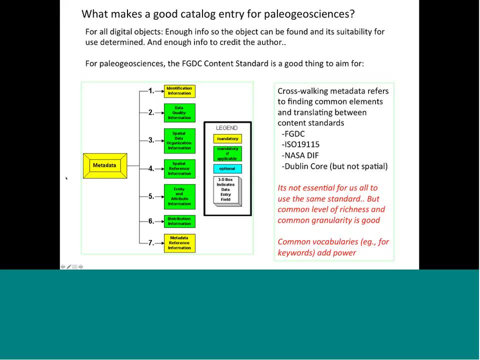 for data quality, two elements related to the spatial data organization and the reference. there is information related to entities and attributes, what was measured, there's information on the distribution of the data, how to get the data and there's information on how the meta-data was created. so there are many different standards. FGDC is only one and 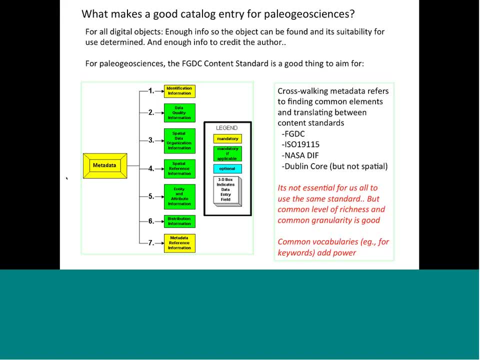 crosswalking metadata refers to finding common elements and then translating between different content standards, such as FGDC, ISO 19115, the NASA DIFF standard and Dublin Core, although Dublin Core, and its skinniest version, does not have spatial information, so it's not essential for all of us to use 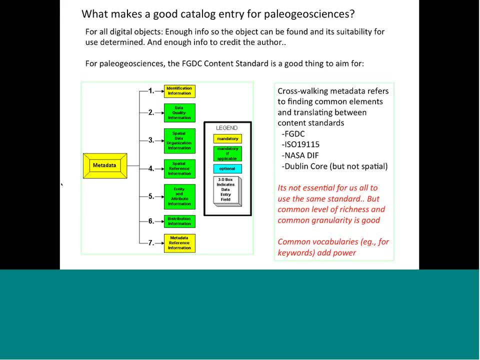 the same standard, but a common level of richness and common granularity is good. in other words, if some of us decide to have a level of richness that includes keywords and some of us do not, this will make a distributed or shared catalog less useful. it's a level of richness varies from one provider to another, and then we'll look at that in the next slide. 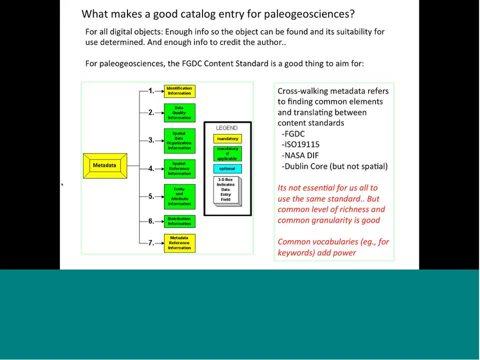 Likewise, if some of us describe data sets at a collection level and others describe data sets at a very fine sample level, that makes the combined catalog less useful. And then, finally, as a goal to reach for in developing these interoperable catalogs, the 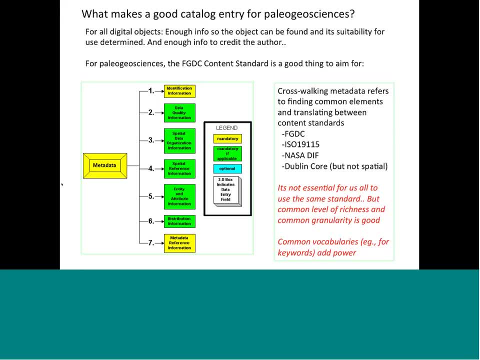 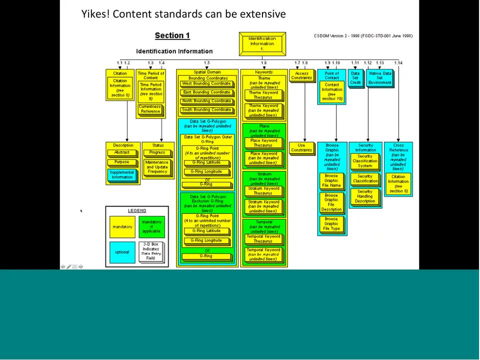 use of common vocabulary, for example, a philosophical keyword, adds power to the distributed catalog that we're trying to create. So this is a scary figure showing all of the different fields associated with section one and the F2DC content standard, And so some of these content standards can be extensive. 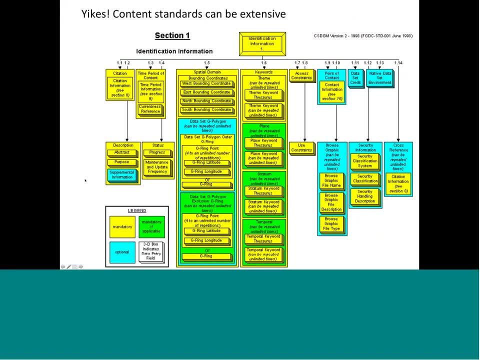 And at the World Data Center, we have tried to draw a kind of a happy medium between the level of detail that we can achieve and the number of data sets that we are able to archive, Because, in addition to being reasonably complete with our description, we also want to archive. 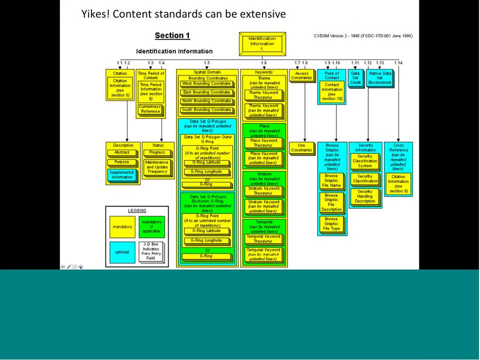 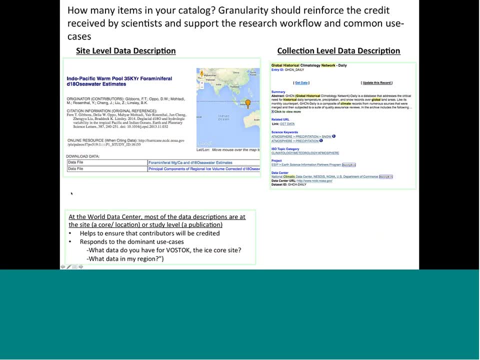 for as much data as we can. So one of the other issues in developing a catalog is what level to identify items, or in other words, what level to make the catalog entry. So on the left here is a site level catalog entry for the Indo-Pacific warm pool seawater. 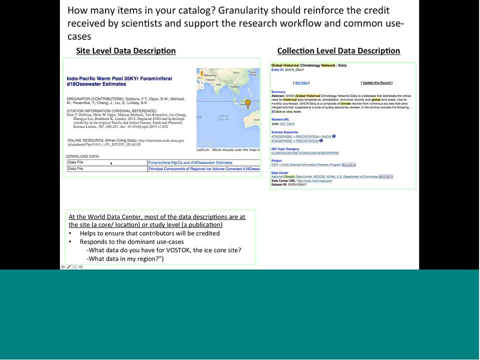 O18 estimates. So, in general, the data archived at the World Data Center are at this site level. In other words, they're at this site level. In other words, one data set description refers to a single site or a group of sites associated. 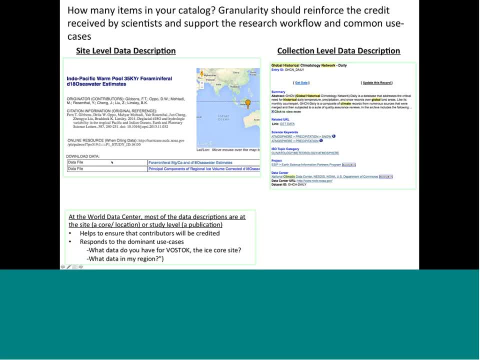 with a publication. On the right is an example of a collection level data set description from the NASA Global Change Master Directory. So this is a collection of global historical climatology network consisting of maybe 3,200 different sites And because it's a collection level record, the individual site location is not shown. 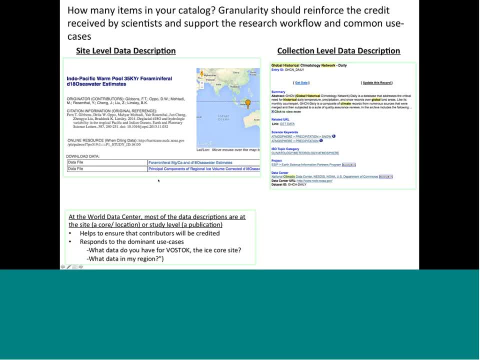 It's not mappable. So just to reiterate, at the World Data Center, most of the data set descriptions are at the site level corresponding to a coral location, or a study level corresponding to a publication, And we have adopted this level of granularity because it helps to ensure that the individual 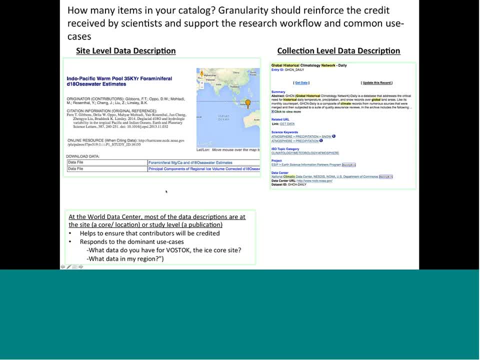 contributors will be credited And it responds to the dominant use cases that we get, such as: what data do you have for Bostock, the ice core site, Or what data do you have in Monaco? What data do you have in my region? 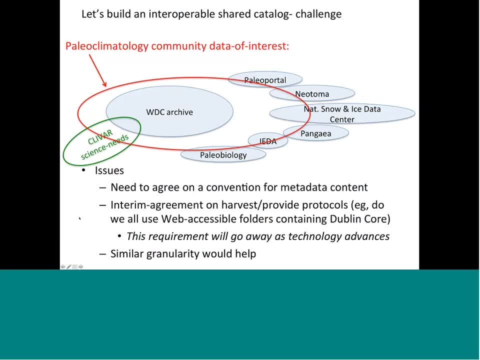 Okay, So I want to talk a little bit about my vision, or my idea of building an interoperable shared catalog and where the challenge lies. So what I am hoping is that all of us data providers can build a catalog that harvests catalog elements from other catalogs in order to meet the needs of our user community. 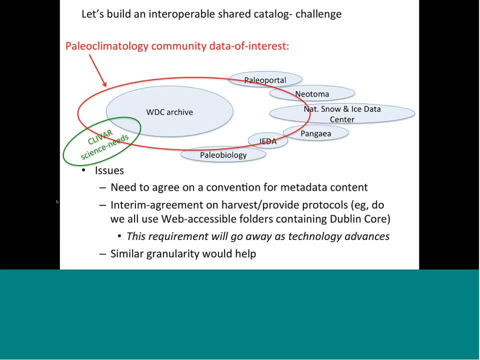 For example, for the paleoclimatology community that I serve, the data set description is very important. The data of interest for my users includes probably all of the data in the World Data Center archives and probably some of the data in Paleo Portal, some of the data in the paleobiology. 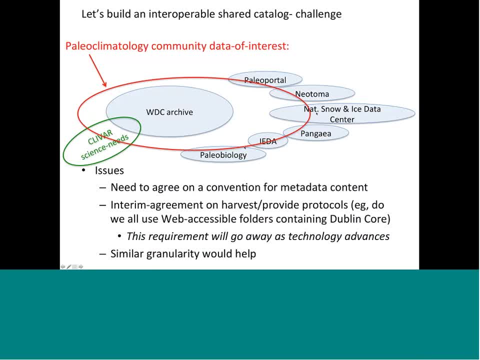 database that we just talked about and some of the data from the National Small and Ice Data Center. In fact, my user community might hope that I would harvest some data set descriptions from CLIVAR, the Climate Variability Study, in order to make this catalog of elements. 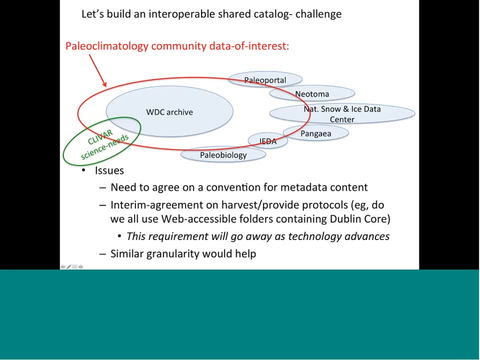 Okay, Thank you. Thank you, And I do hope that we have a model of this one that's bounded by the red line that they see, And, similarly, CLIVAR might harvest several of the records from the World Data Center that have specific climate variables reconstructed, such as precipitation and temperature. 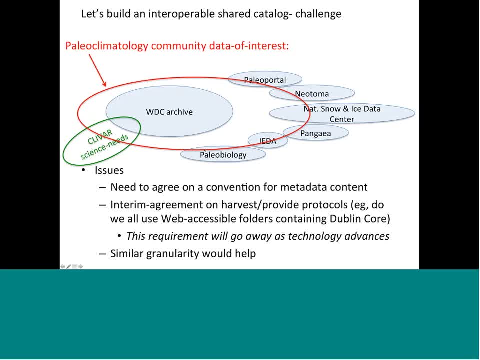 And similarly, paleobiology might want to harvest several catalog descriptions from the World Data Center. So some of the issues in achieving this interoperable shared catalog are that we need to agree on a convention for metadata content, need some interim agreement on harvest and provide protocols. for example, would 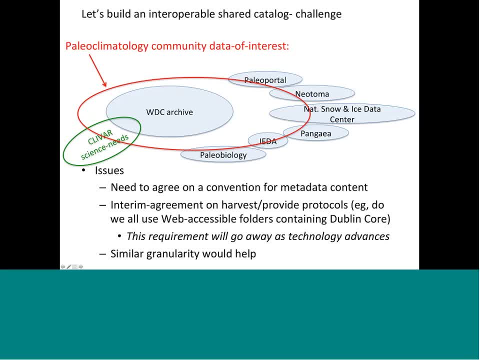 we all agree to use web accessible folders containing Dublin core metadata as a content standard. this agreement will go away in the future as technology advances, but right now we wanted to implement an interoperable data catalog. tomorrow, making some of these agreements will help this. does it help the library? 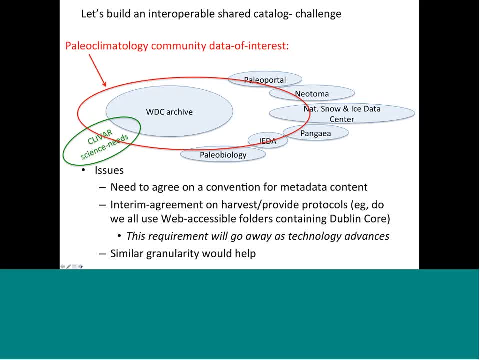 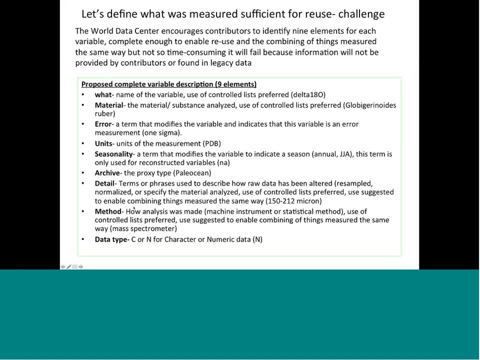 community and then, I think, similar granularity recall. okay, I think the last challenge I want to describe is our effort to encourage the community to identify better what was measured, and so we are focusing on nine elements that we think are standard for each variable. now we're going past the metadata to talk. 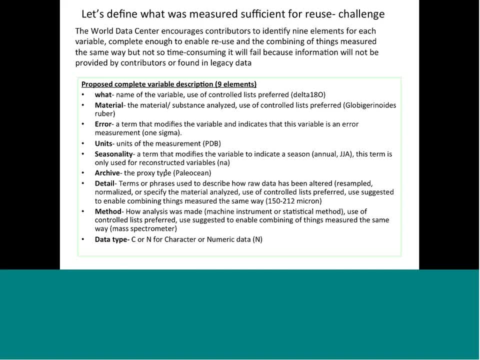 just about. when we receive a time series or a measurement, what things do we need to know so that to enable reuse of that measurement and enable the combining of things that were measured? in the same way, we think we need to know what the measurement is, what material it was measured on. um, we have an error quantity here that. 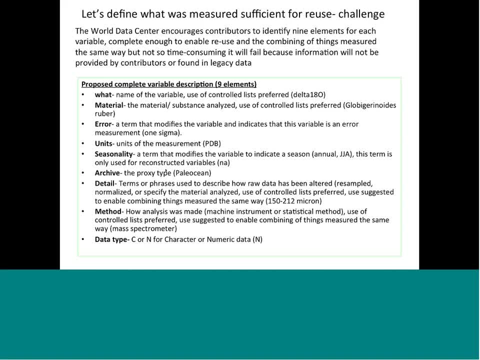 identifies whether this variable is an error term or not. we need to know the units. we also modify these very well. there is a particular seasonality that was reconstructed. we identified the arc arc- arc I according to one of these 18 different proxy pipes. we have a category for. 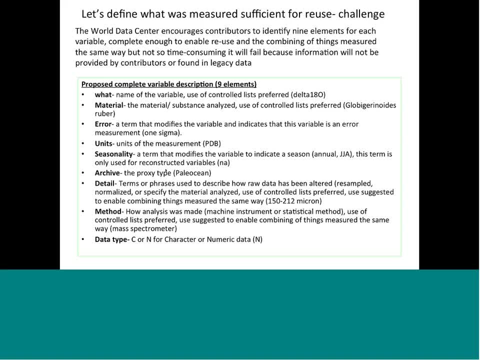 detail, which includes terms or phrases used to modify or describe how the logic is altered, resampled or normalized or specified, whether the certain material of a file fraction 150 to 212 micron. we need information on the method, how the analysis was made and, to make it machine readable, we need to know the data type. 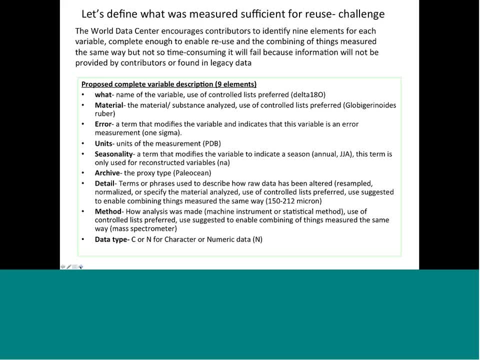 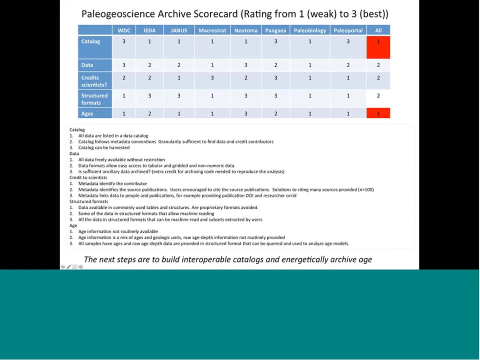 whether it's character or numeric, and this is kind of evolving. I think this is really the difficult place right now for all the different archives is to agree on what level of detail is needed to identify what was measured. okay, my last slide is to give you a scorecard on 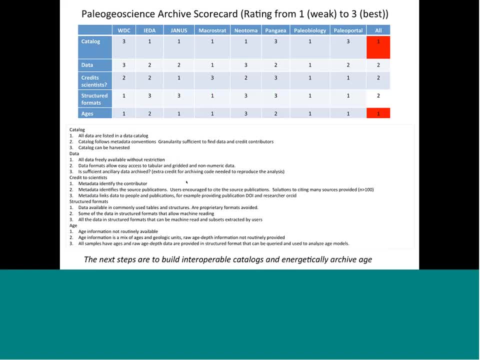 how we're doing. so what I've done here is to look at a couple of different aspects of maturity for the different period of Geosciences archive, and this is just off the top my head for discussion looking at how we're doing, how I use data: Janice macrostrat, Neotoma Pangea, paleobiology, paleoportal and some of the 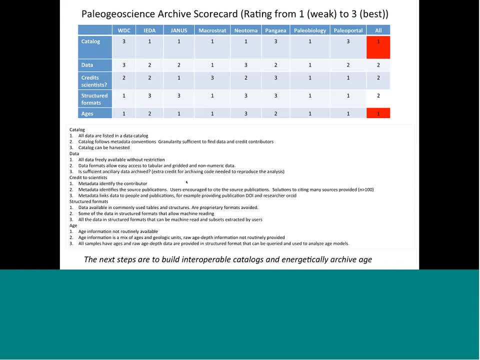 other data archives that are discussed in the webinar series are doing in five different categories. do they have a catalog? can that catalog be harvested? and I've scored these one to three, from weakest to best, looking at whether the data are freely available and whether sufficient ancillary data is archived. 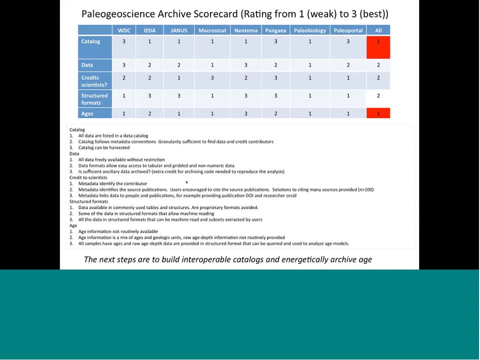 looking at how they credit science, looking at whether they structure the data and looking at how they treat agent for making. and I just want to point out for now that there are two weaknesses, I think, as we look across all these different archives effort, and one is that 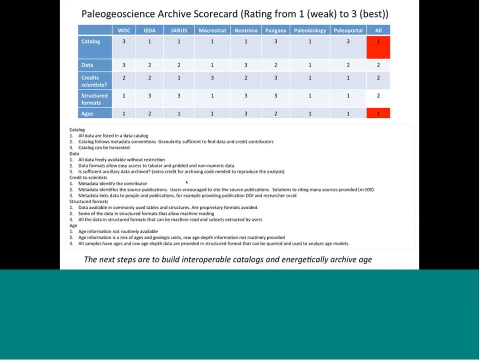 we haven't yet achieved this interoperable shared catalog, and so I've highlighted that in red and then second. we've been our standard, and our efforts in archiving age information has varied as we've gone through time. I think all of us would agree that the holy grail is to have sufficient age. 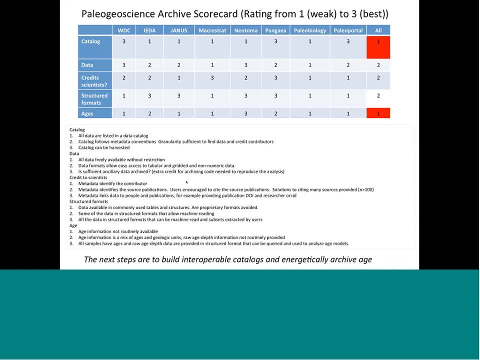 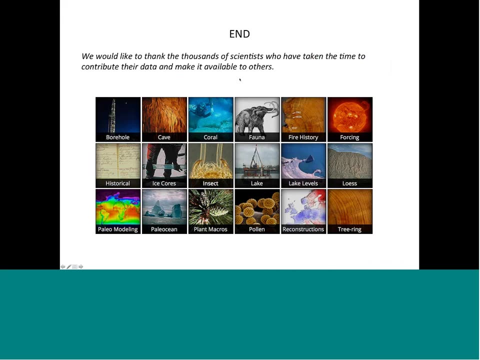 information that we can redo, age models and on. in many cases we haven't collected enough information to make that possible, so I think I'll stop there by thinking. the thousands of scientists who have taken the time to contribute their data and make more others and take questions. 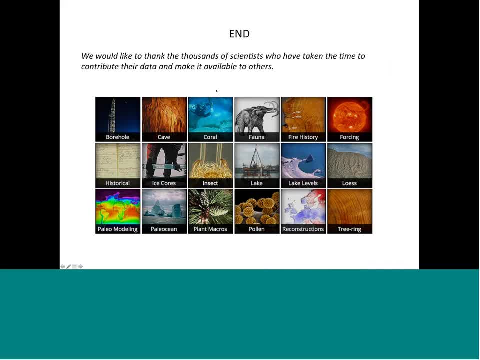 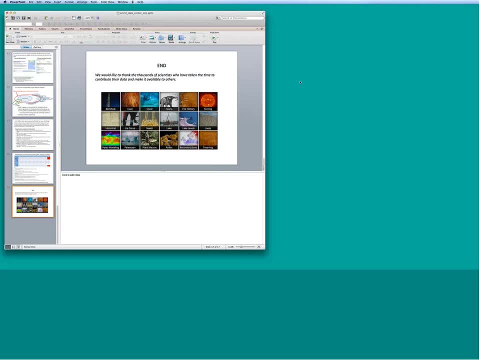 from the audience. Dave Leslie, I'll go ahead and pass to you for questions. sure, thanks, Dave. um, okay, related to this last slide. the first question is: who puts the data into the structured data file and is it hard to make people use it? yeah, this is a really tough question. so right now we are. 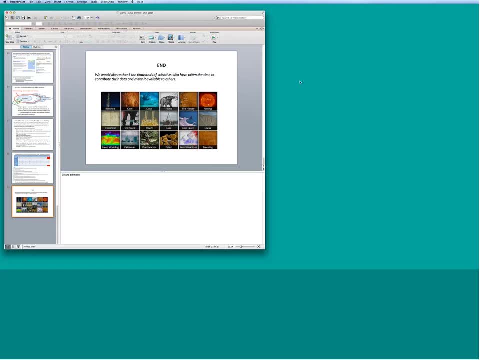 trying aggressively to structure the data for the community. so, um, you know, October 2013, we're trying to do a lot of work to build the structured data, and so we're really interested in what we can do in the future along. the main topic is: everything is structured, and so what we're trying to do is we're trying to 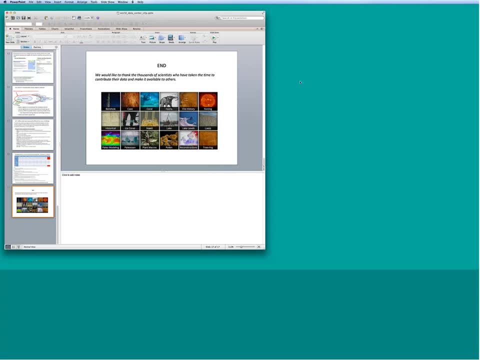 initialize the data structure and also try to do this with all of the world's paleo climate data. so what we're trying to do is a gradual evolution where the effort to structure data files and really the structure that's selected by that they would like to see. yep, okay, thanks. the next question: do you have any? 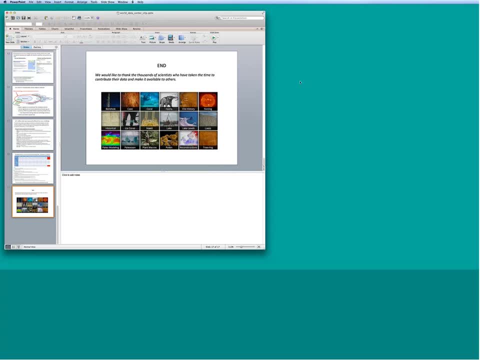 challenges dealing with very large data sets or ongoing continuous data sets. uh, we might have to refine ongoing continuous, because I'm not sure what was meant there. we, we do, for sure, receive updates to data sets, that's, that's routine. the metadata identifies the updates, so that's straightforward. large: 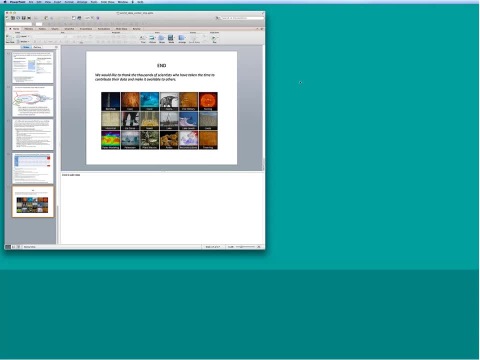 data sets. we're lucky because we're part of NOAA, which is a satellite heavy organization, and NOAA is used to dealing with very large data sets, so theoretically we've been able to piggyback on NOAA resources and NOAA solutions for archiving large data sets and archive in that way. archive transit. 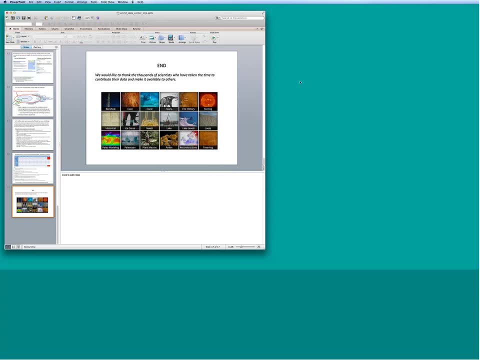 model simulations and other data. okay, continuous data sets. um, what was meant was sensors that are continuous and continuously collecting data. I think you addressed that by the updates to existing data sets, right right there? yeah, to try to elaborate a little bit, there is a loose division like: what is the in the world of climate data? what is? 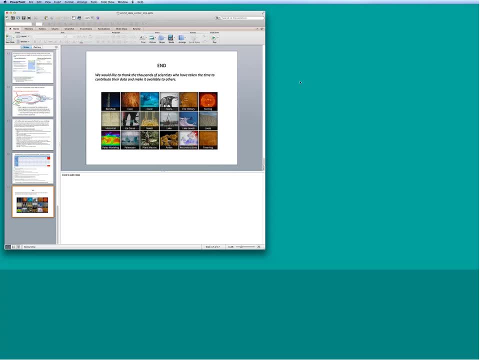 the core view or what is the mandate of the World Data Center, data center, data center and in general. we do not archive uh modern monitoring data unless it relates to calibration of failure samples, and we do not archive instrumental data. the World Data Center's mission is to archive data derived from 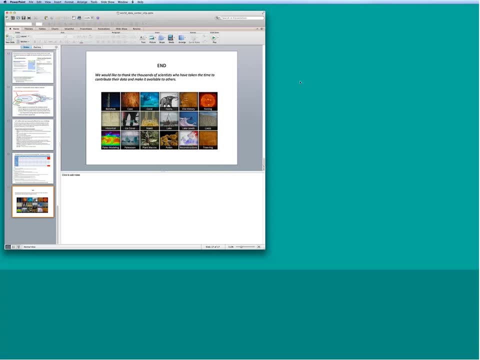 paleo proxy measurements, including historical records such as Ben Franklin's Diary. okay, great. the next question is: can you explain more about how you maintain your keyword list? I think the question was to explain how we maintain our keyword list. we are, our keyword list is very immature. um, we branched off from a NASA global change. 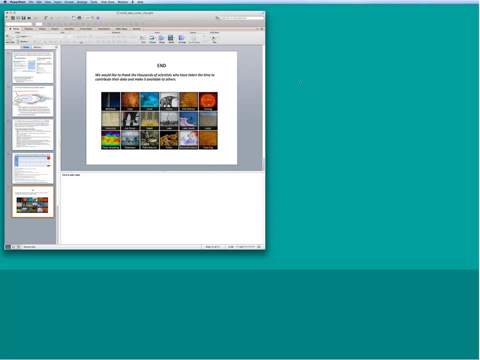 master directory thesaurus for paleo climate data. we modify that to associate keywords with 18 different proxy types, but we are really eager to work with the research coordination that we're working on right now. so I'm going to go ahead and show you a picture of the application network for paleogeosciences and, at the 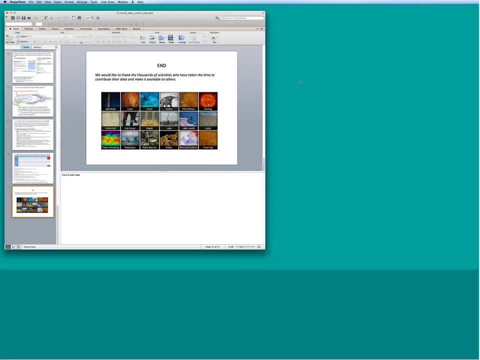 end of our two-year effort, I think that we'll have a much better and sturdy set of keywords and a sephora for everybody to use, and I don't think we have that now. next question is: given how popular the topic of climate is among non-scientists, 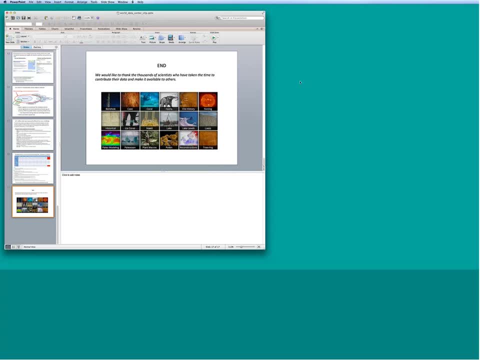 is there an effort to help beginner non-domain users or help them use the data correctly? Yeah, There are several approaches to this. The most fundamental approach for many people delivering things over the web is an approach called laddering, where you try to provide. 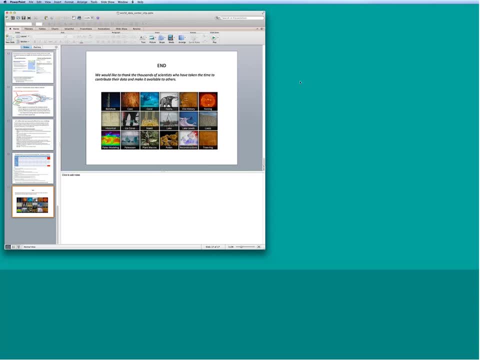 relatively easy information, kind of low rung to the ladder where any user can get on and kind of see what's going or understand a topic And then later they can go up the ladder toward of increasing complexity and find more refined information, ultimately pointing to scientists. 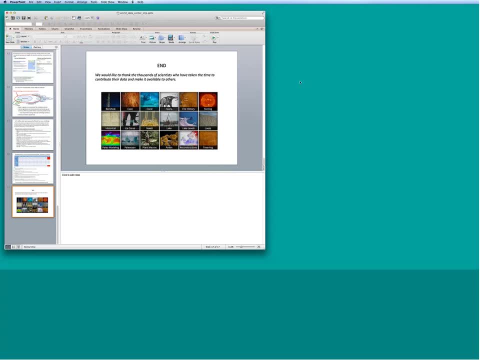 and their data set. So we have tried to ladder information on NOAA themes such as global warming, drought and abrupt climate change and provide both this easy to access information and also, up the ladder, this access to scientists. The ultimate objective in doing this and 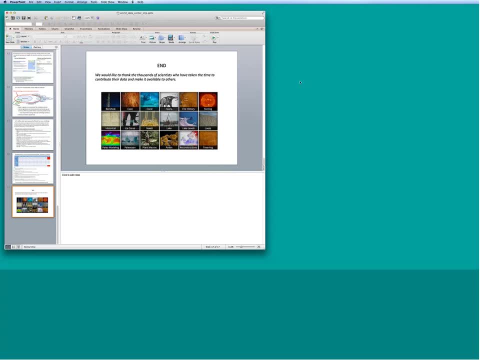 I would encourage all of the Paleo-BioSciences participants and archivists to do this- is to connect data, people and publications, And I think that's going to provide the really rich environment that our users will find most helpful. And so, just to be really concrete here, what we're 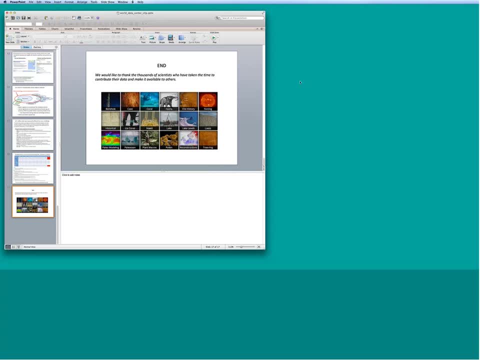 trying to do. when you hit a data set, you should also be able to connect with the ORCID number of the scientist or the contributor and then be connected to that person. Likewise, you should be able to click on the DOI and be connected to that publication. 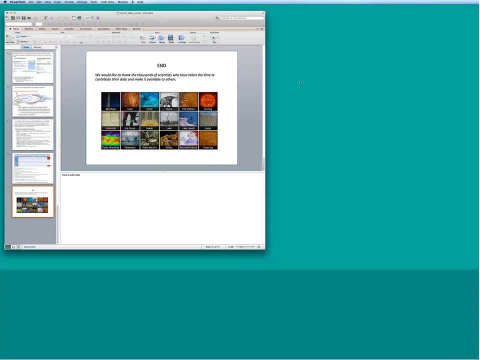 Okay, If we do this right, in a couple years, when you go to a particular investigator, you'll be able to find his publication and his data set, And likewise, when you go to a set of publications, you'll be able to find the scientists and the data associated with that publication. 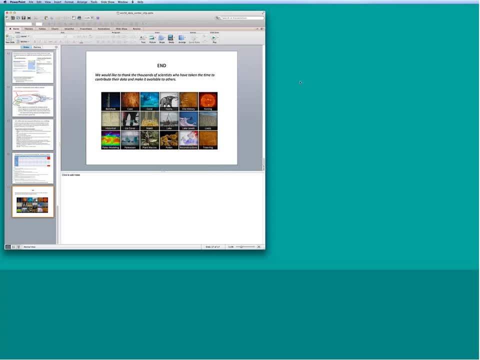 So we are working toward building a really rich network that's going to serve user needs on several levels by connecting data, people and publications. Thanks, The next question is: how do you connect data, people and publications? Thanks, Okay. 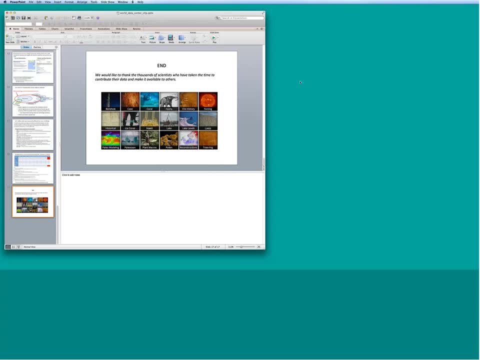 Next question. Well, first a comment. Jack Williams really enjoyed your talk And his question is: what would you say are the immediate actions to take at our May workshop? I'm wondering specifically about agreeing to standards for joint cataloging and harvesting across resources. 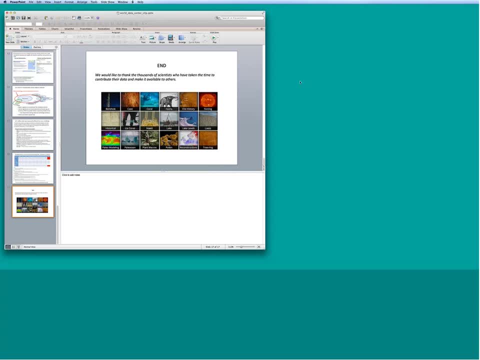 I think that's a great goal and I bet we can do it through the May workshop. I didn't realize that until Mark's talk minutes ago. Okay, Thank you. So I just want to go back to the May workshop, which was the May workshop, and I think that 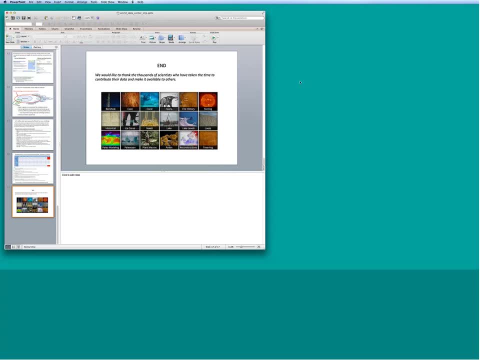 he had an API for us to pick up the catalog descriptions from paleobiology. So that's really exciting and I would say to all of us: we're closer than we think to creating this more operable catalog. So I think that's a great goal for the May workshop. I will 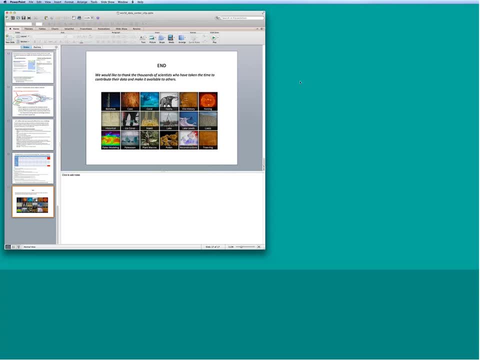 reiterate the other goal that I presented, just because it's such a challenge, And that is, we need to do better at identifying what was measured, And the standard that we should strive is Okay: archive a measurement. we should provide sufficient information to know whether. 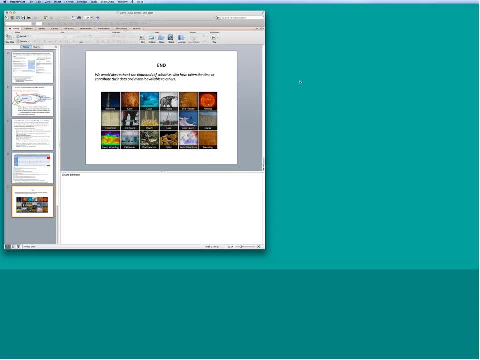 how that measurement was made and whether it can be combined with life measurements or whether it needs to be distinct because the method was different or the some aspect of the sample was different. until we do that, I'm at risk. we are at risk of building a large archive of data where we don't 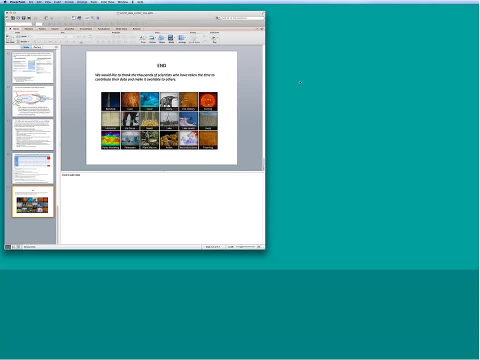 have enough information about what was measured to use that, to reuse that data. radiocarbon is a pretty good example of where they did provide enough information to use the data later. so standing on that as a as a good stepping-stone, as a place to start. 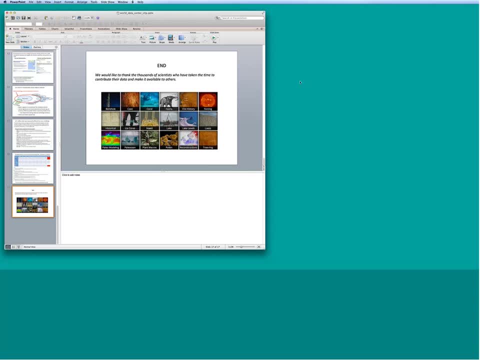 okay, thank you. um, we have no further questions at this time, but you can always send an email to cyber for paleo- the number for cyber for paleo at gmailcom, or either the speakers or the steering committee- and we will be sure to put the Q&A posted up along with this video of the top. so, Doug, thank you asly and also.